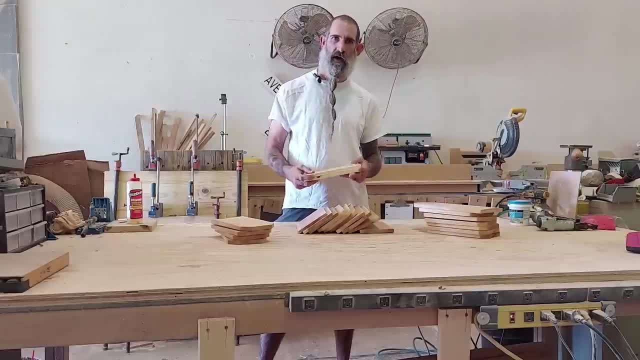 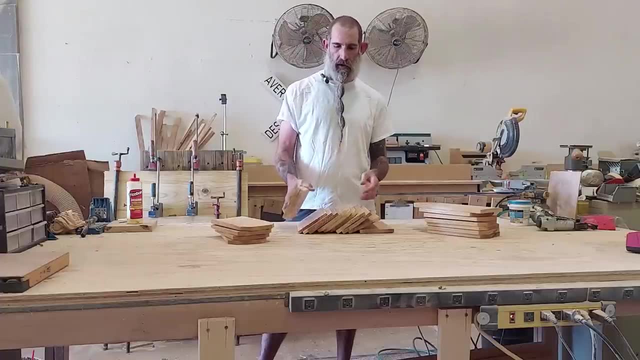 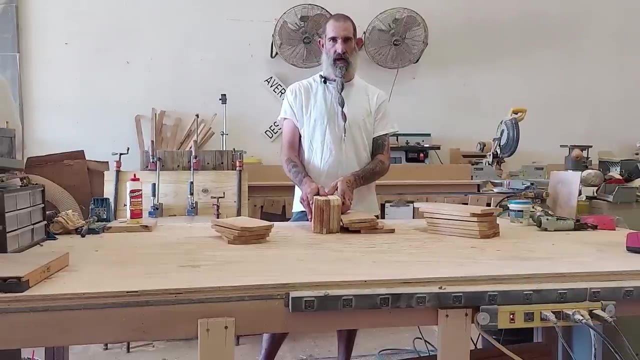 instead of wasting them, we wanted some ideas on how to use them, So somebody responded back with a really good idea: to make a table out of them, and rather than just lay them flat and use seven of them, we're going to stack them on end and use tons of them, So it's going to be a really unique. 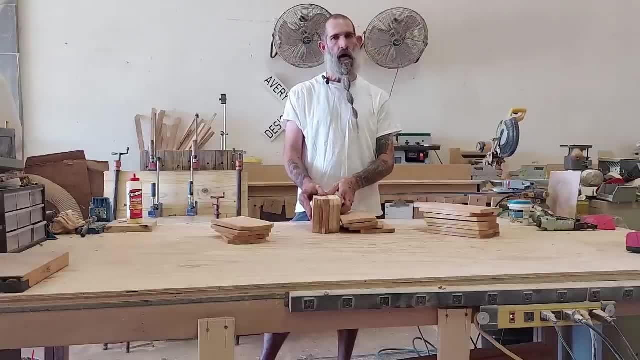 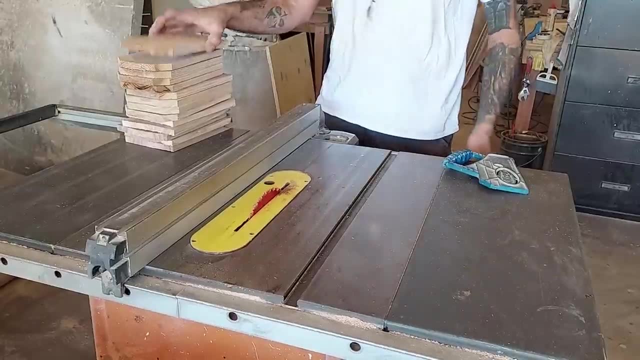 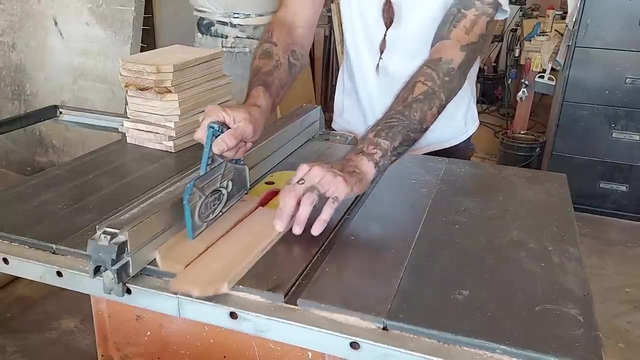 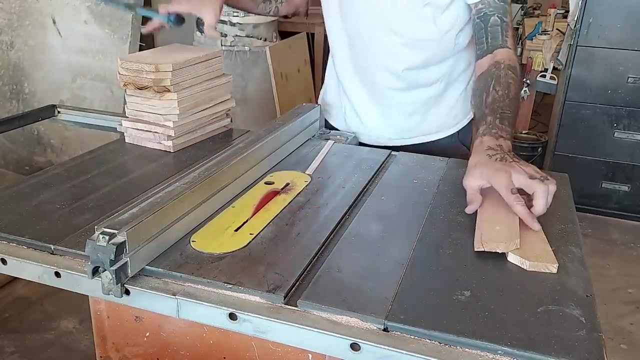 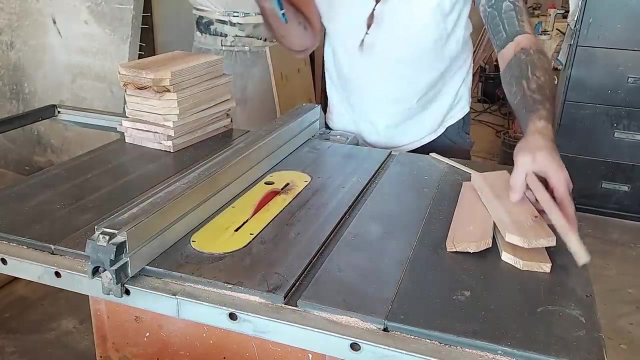 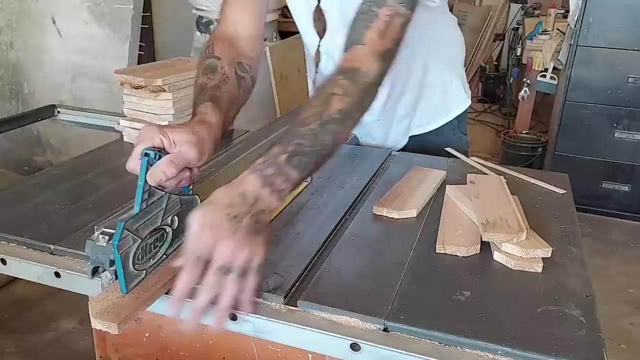 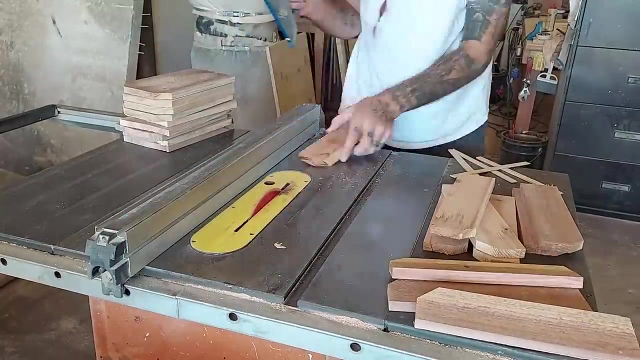 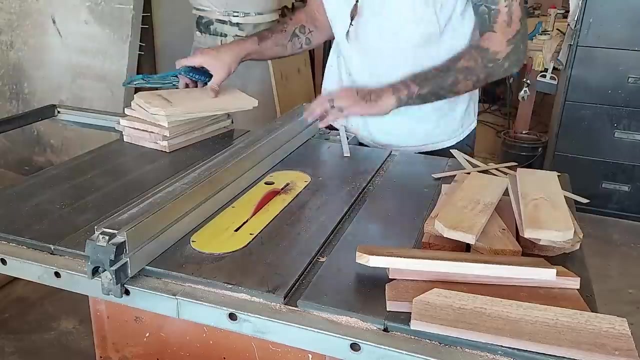 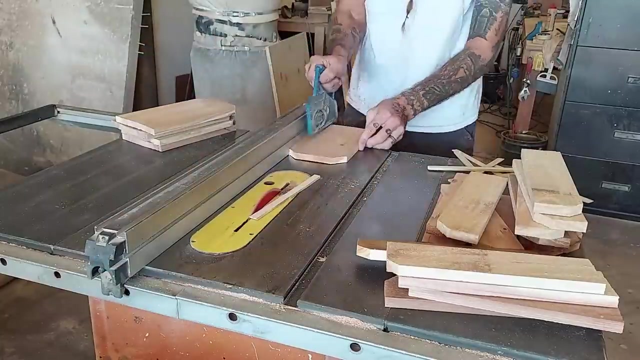 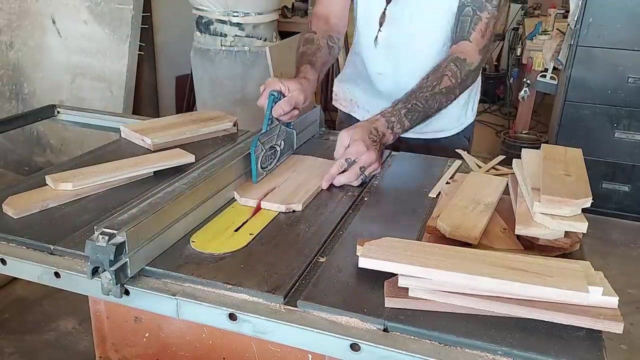 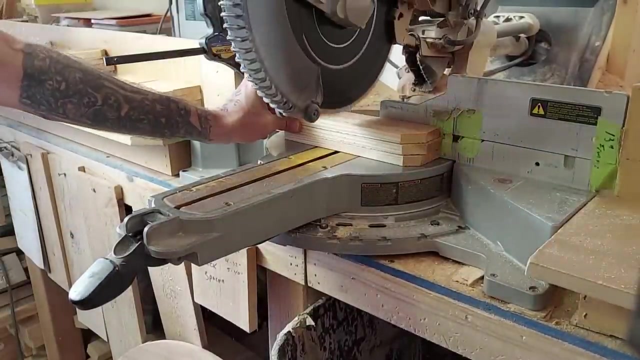 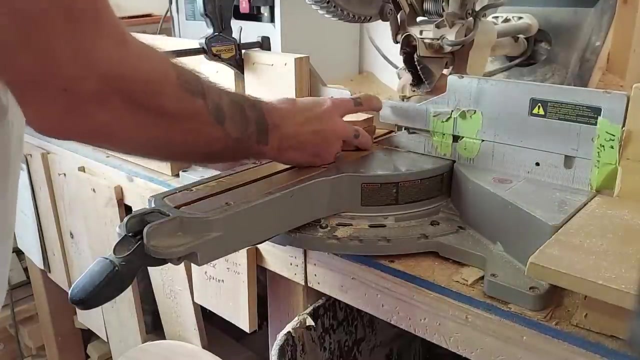 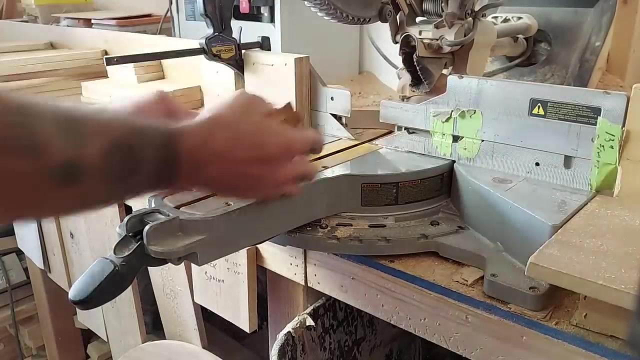 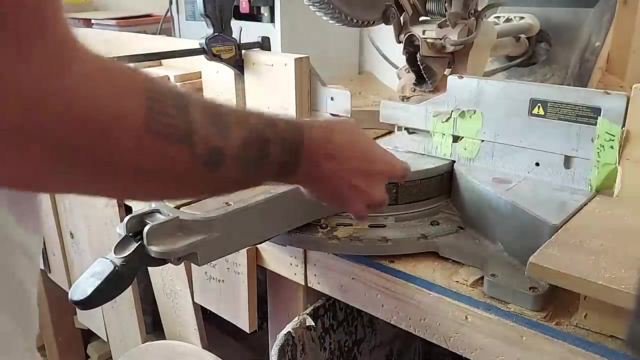 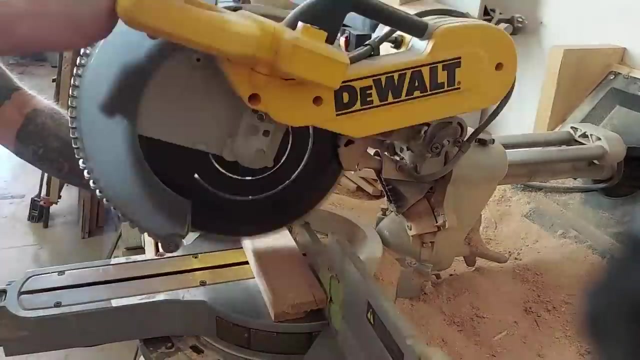 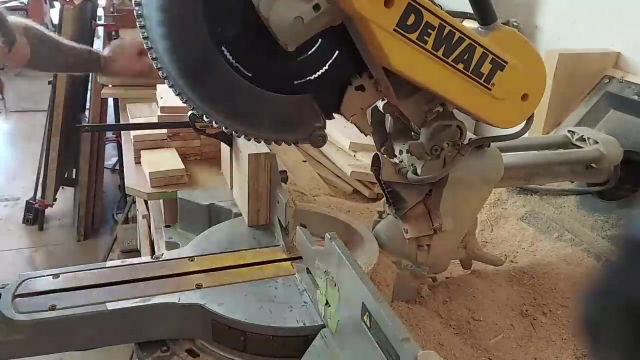 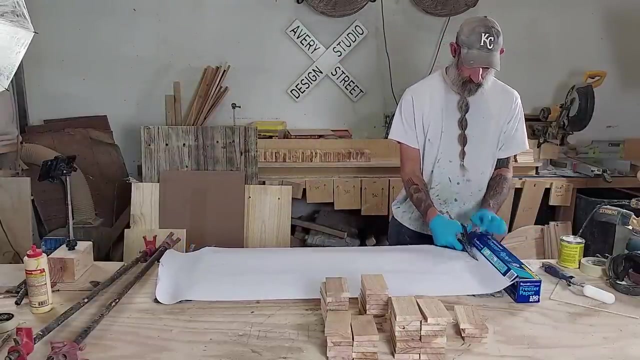 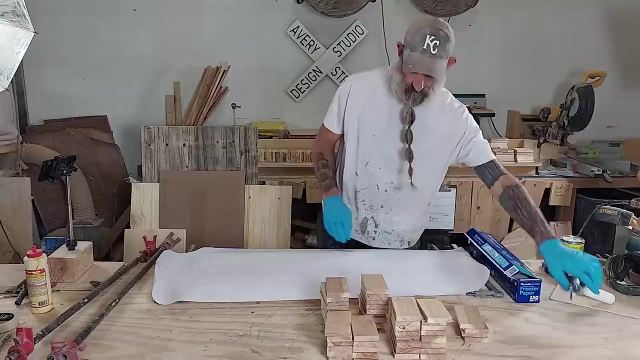 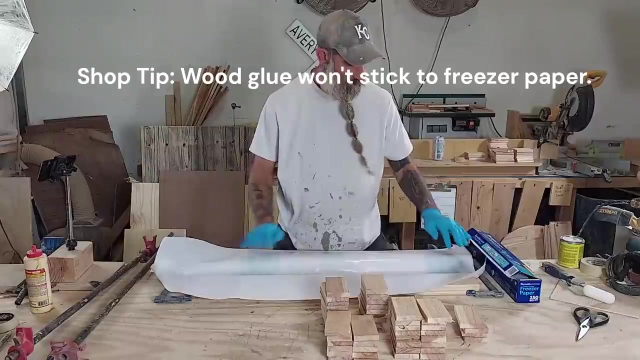 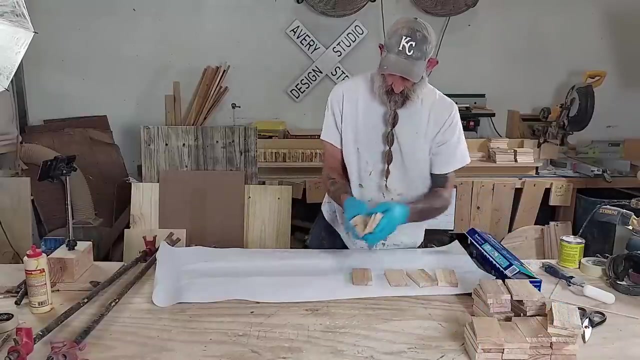 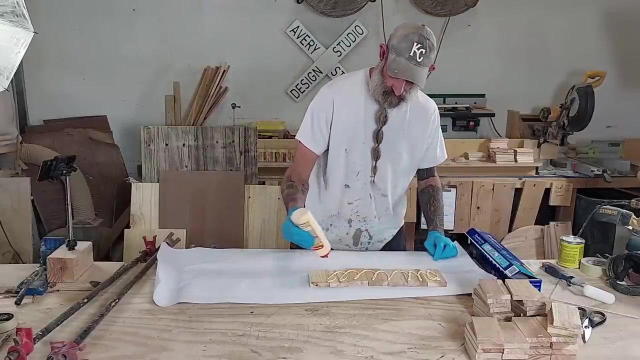 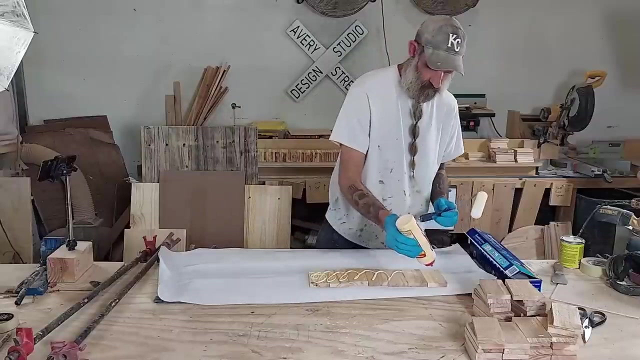 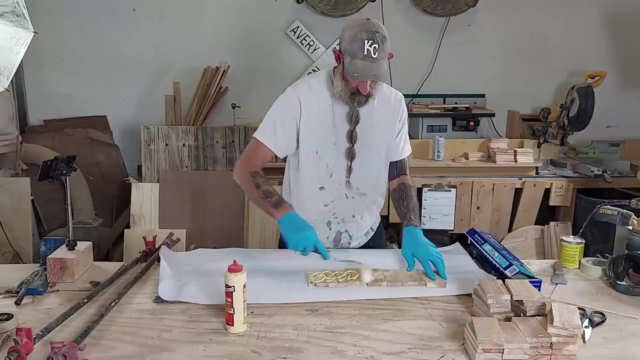 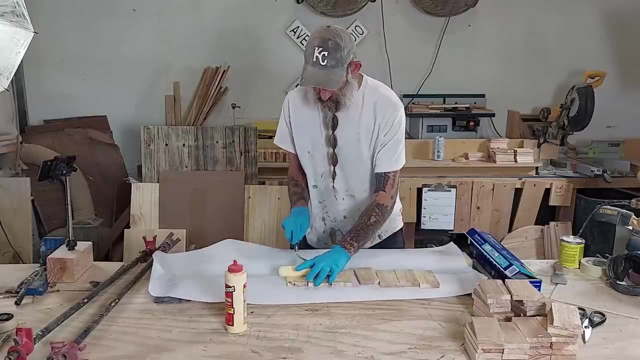 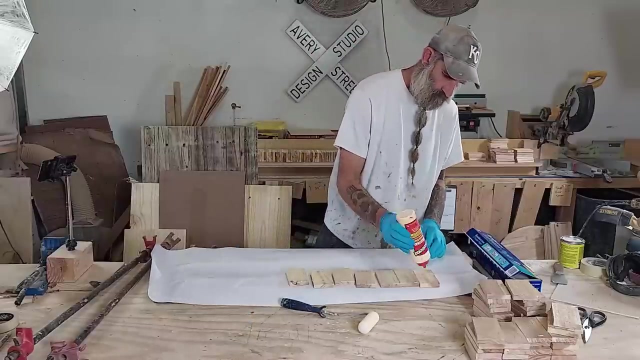 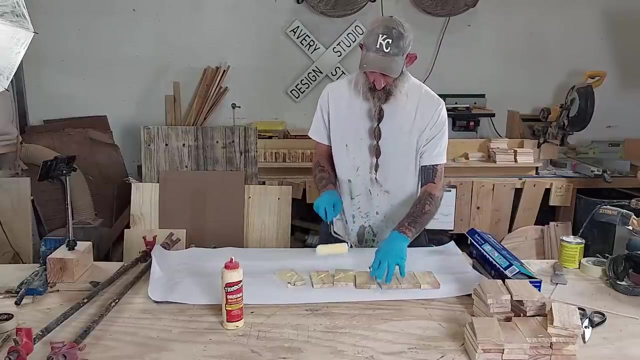 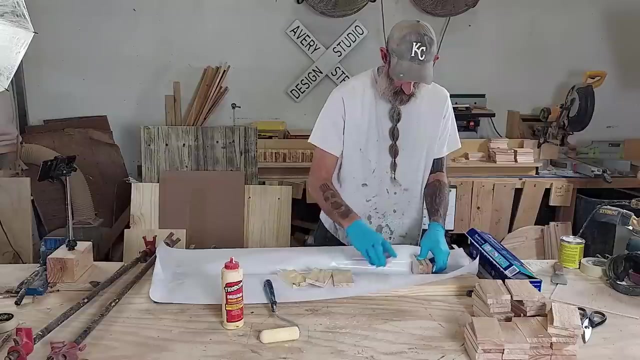 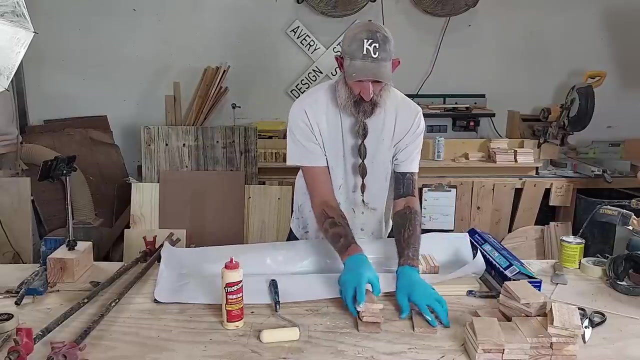 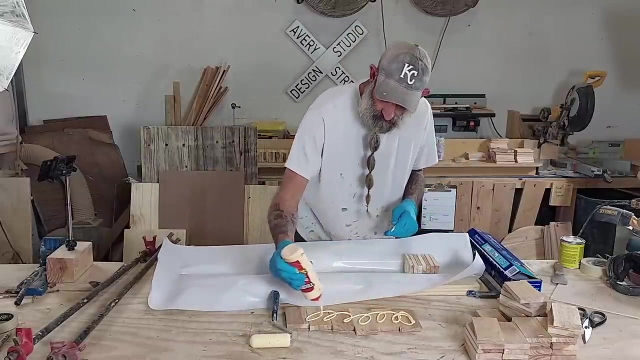 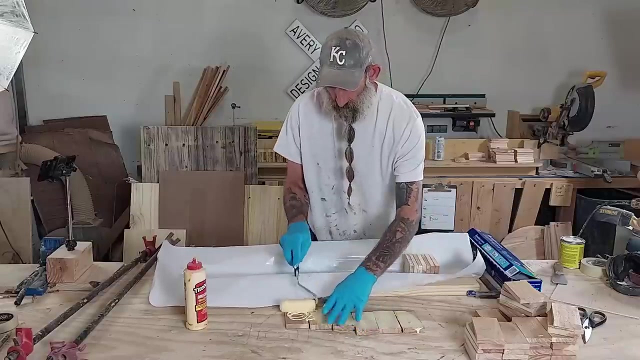 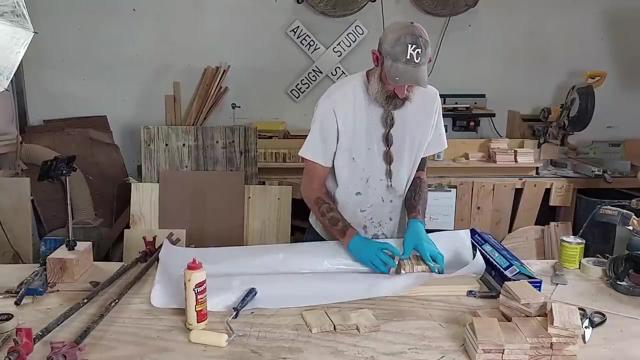 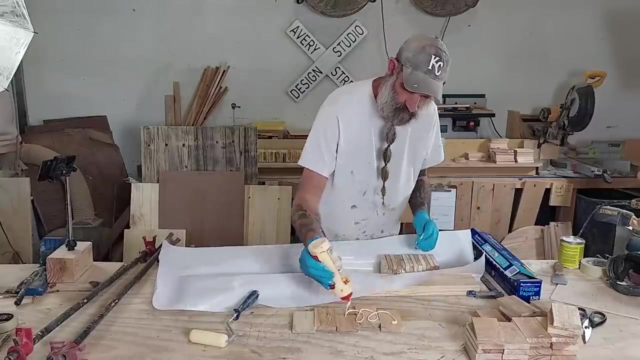 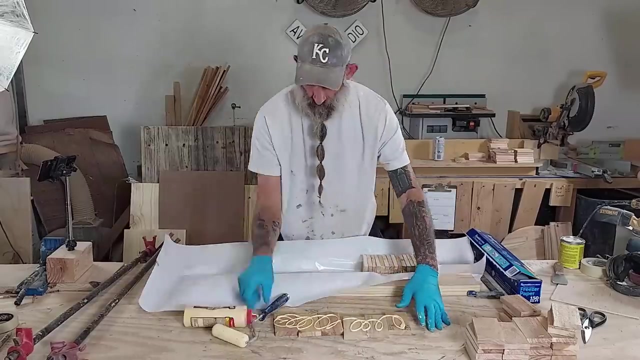 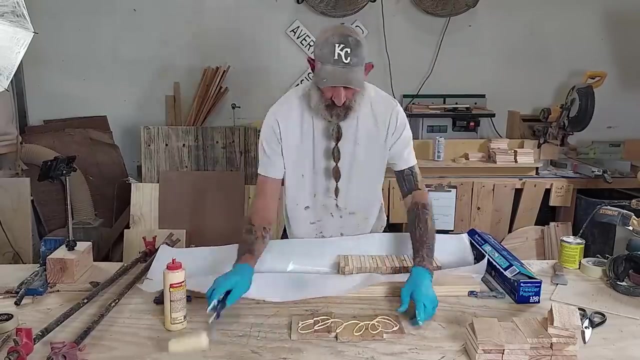 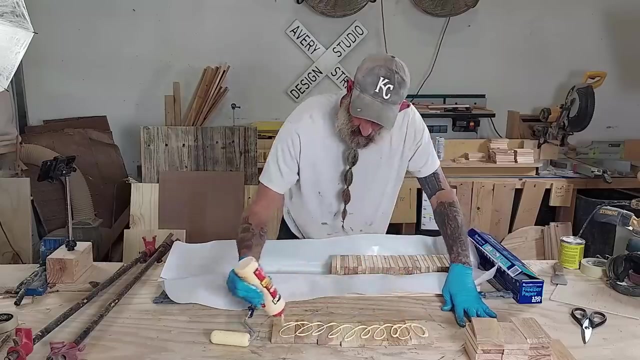 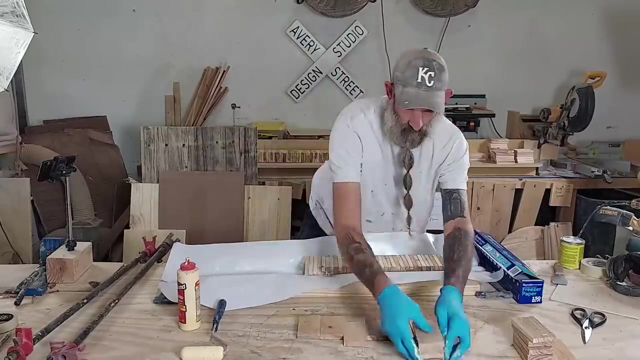 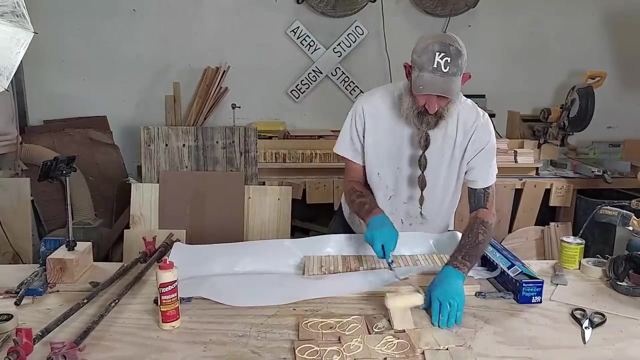 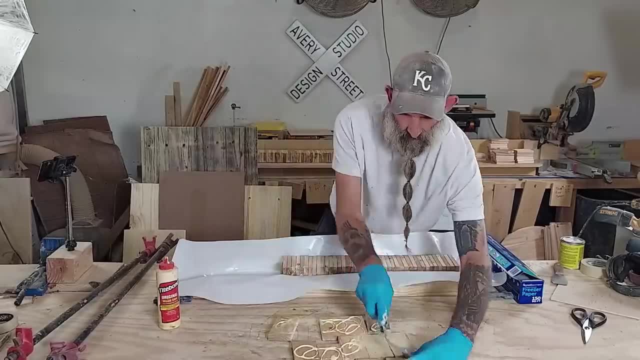 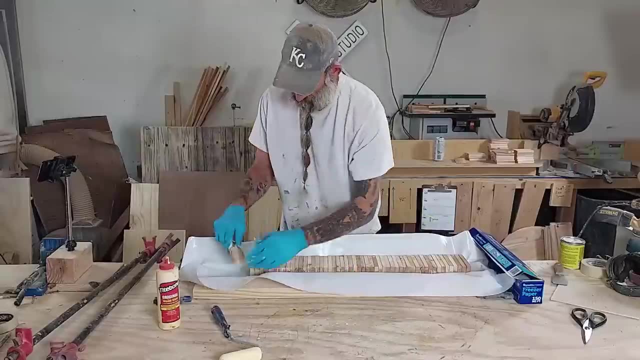 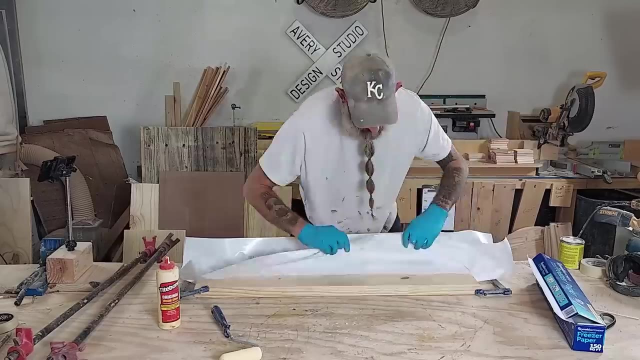 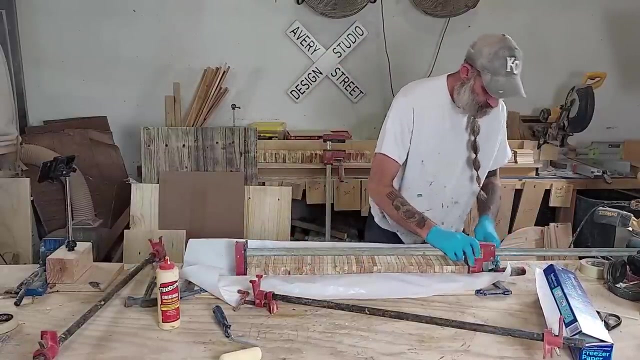 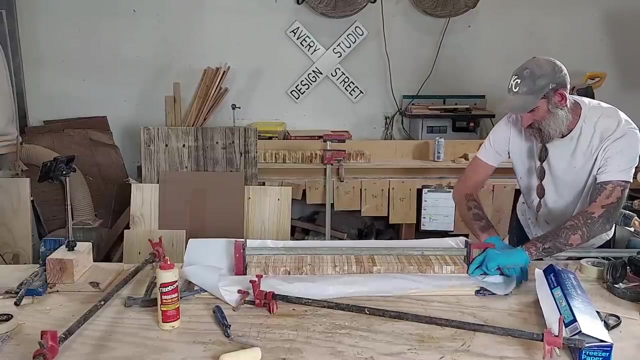 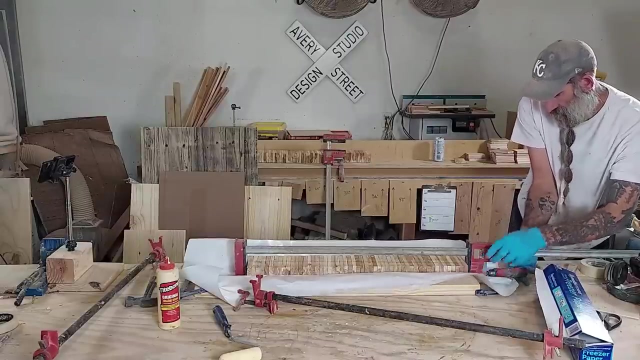 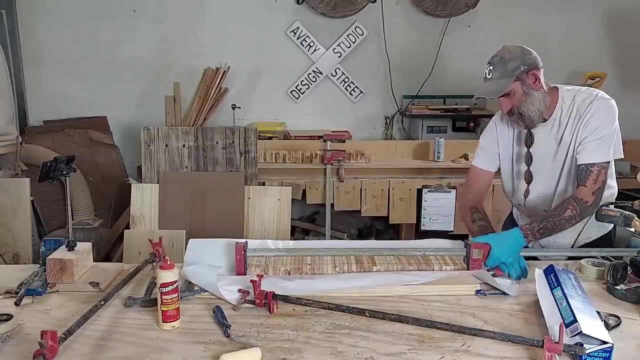 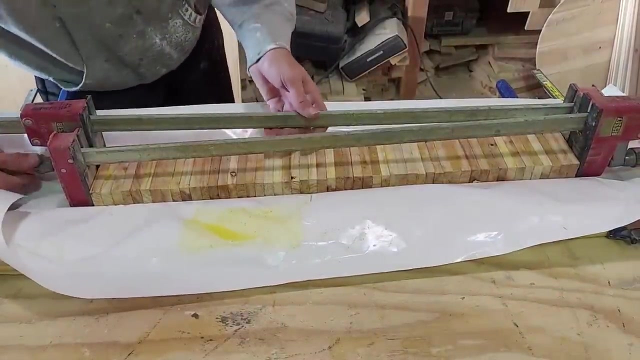 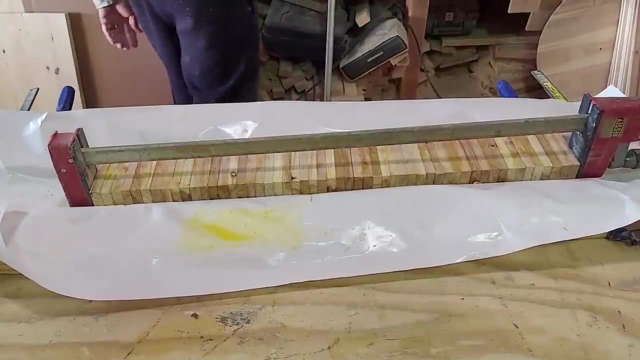 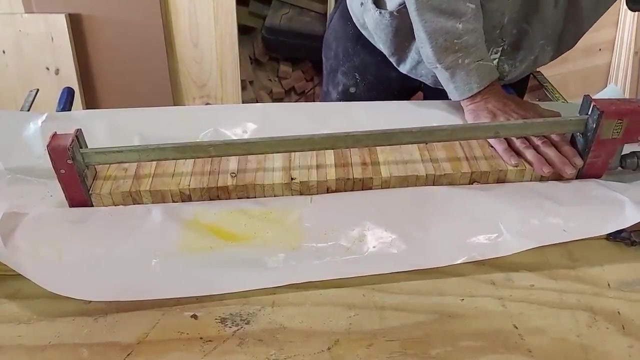 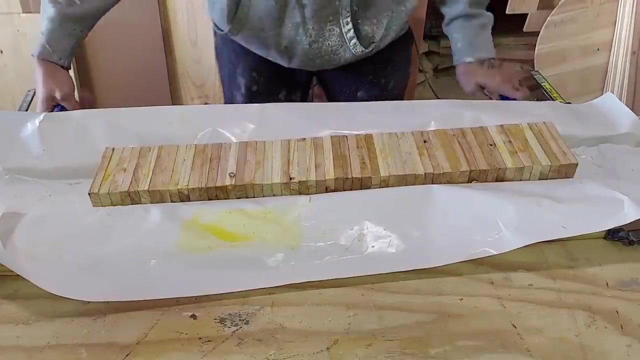 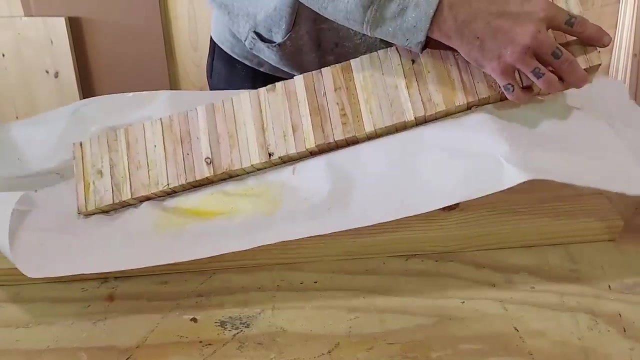 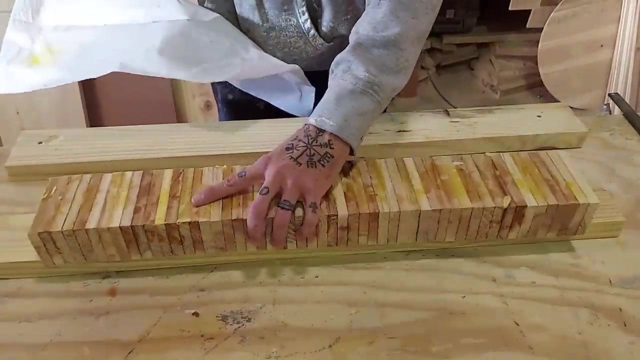 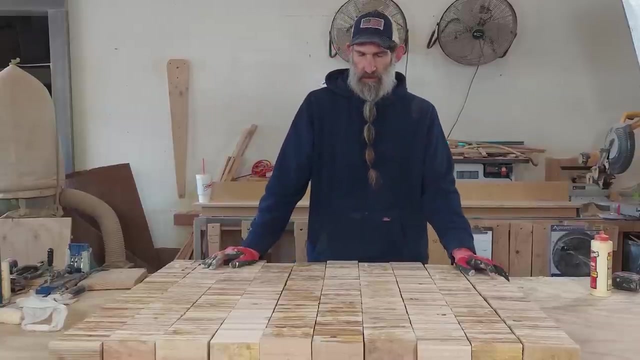 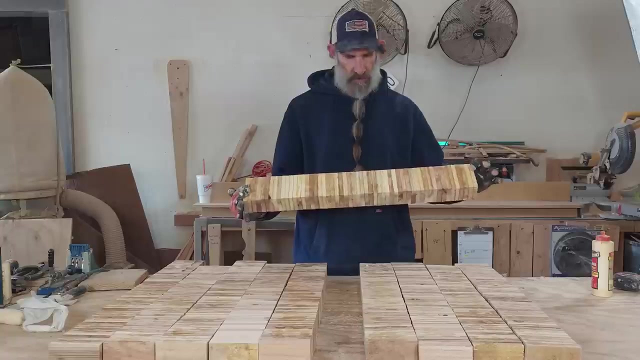 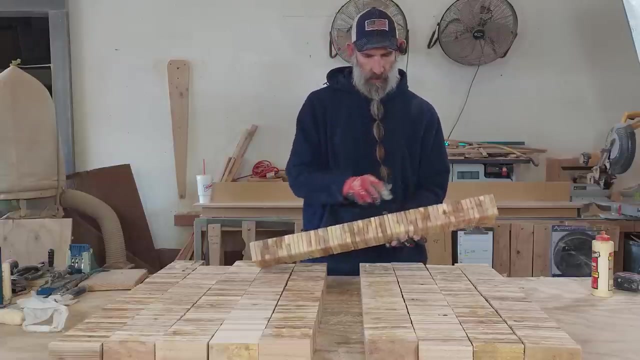 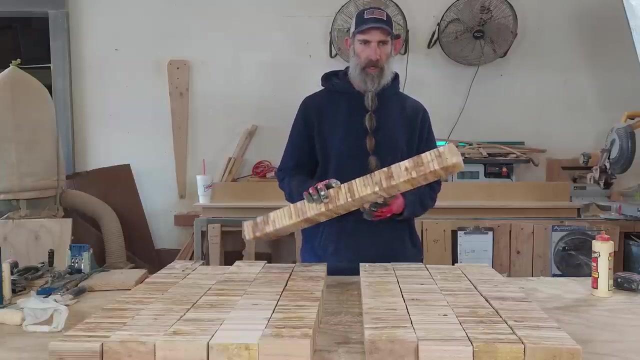 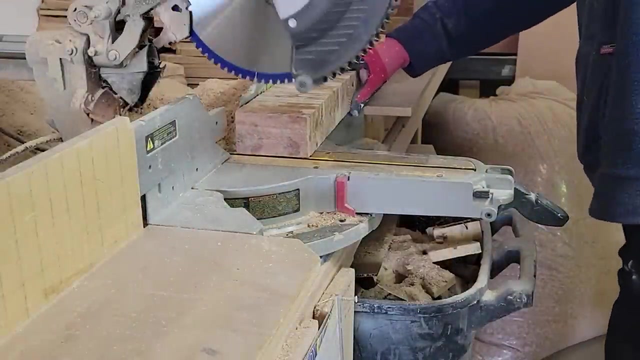 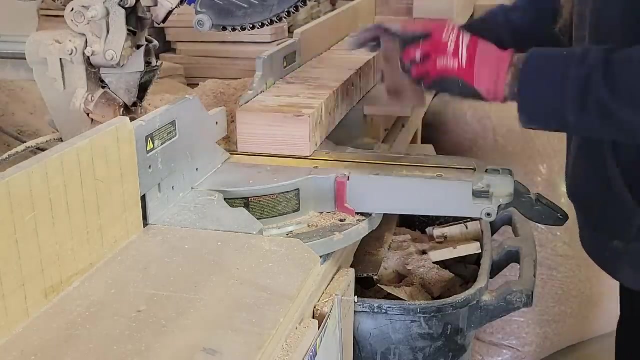 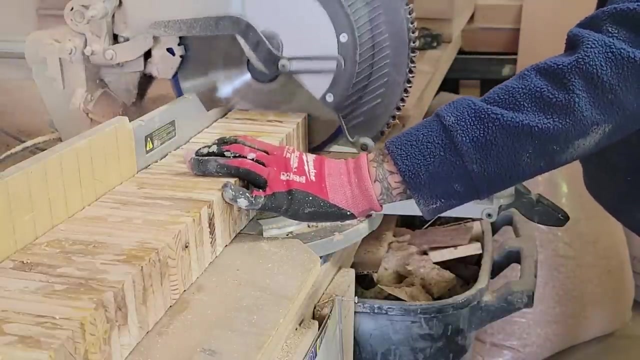 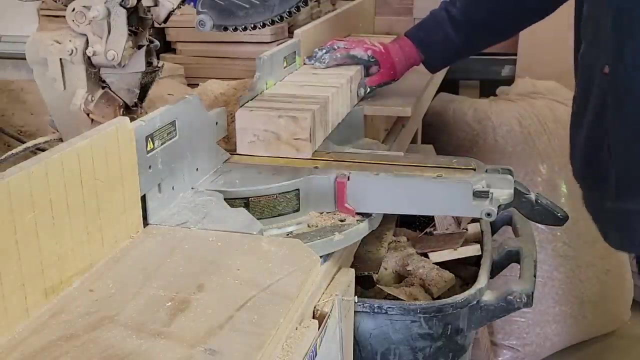 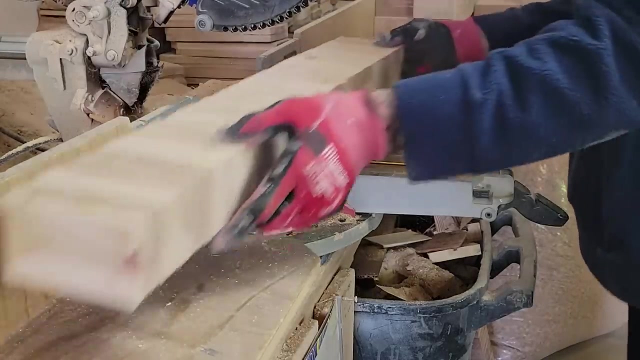 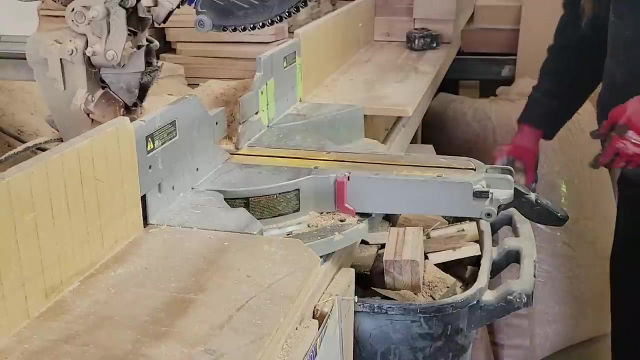 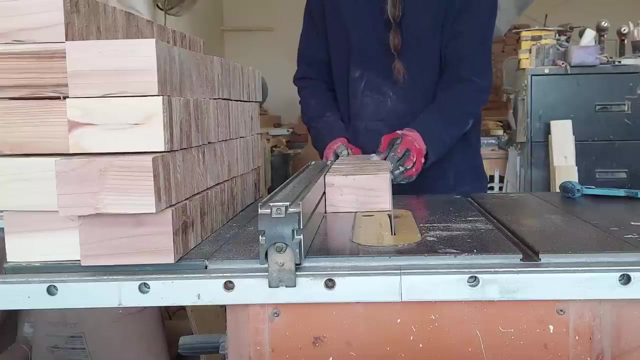 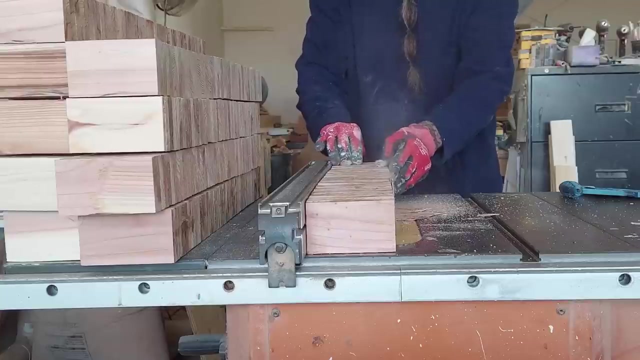 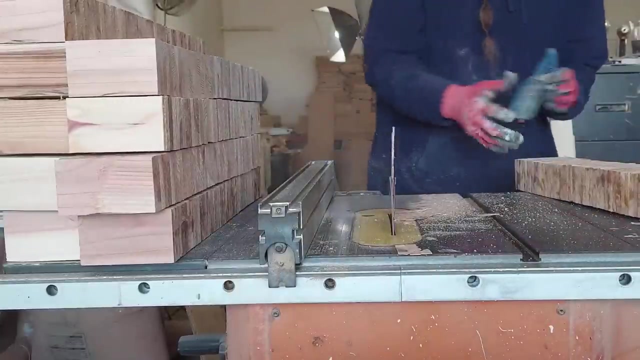 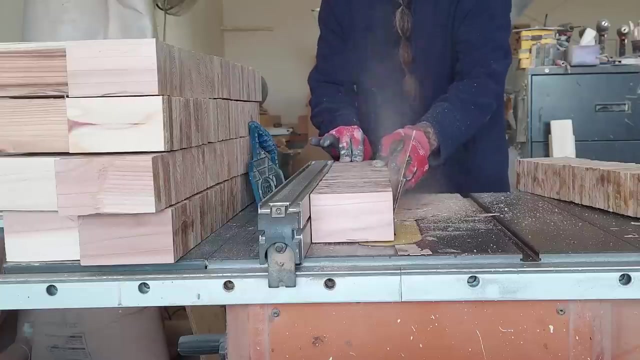 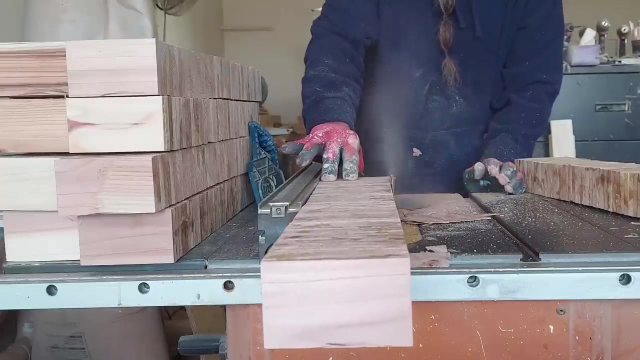 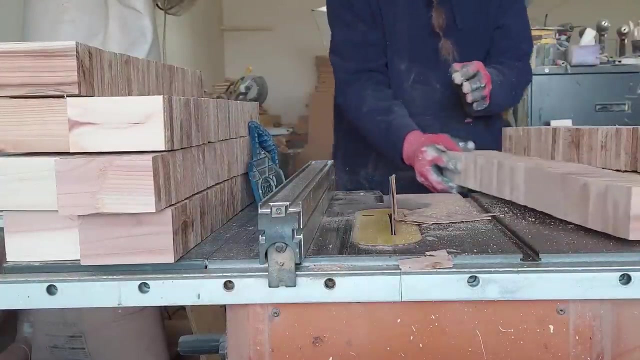 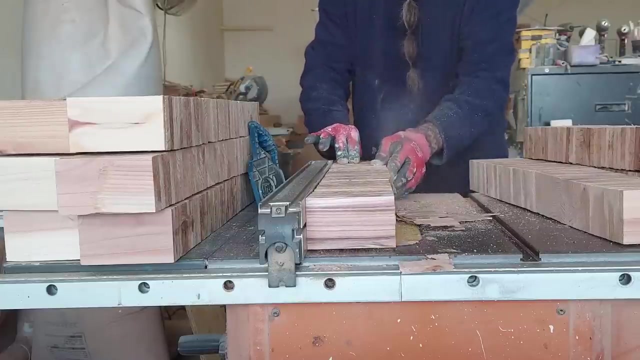 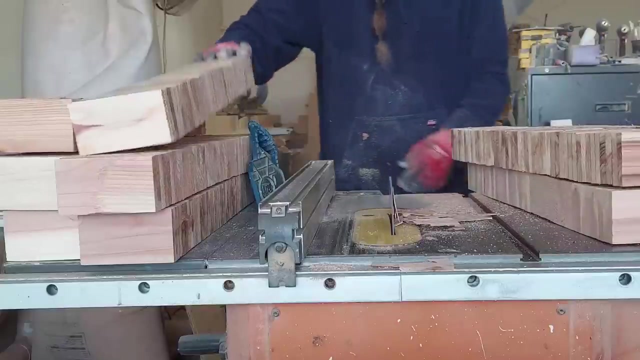 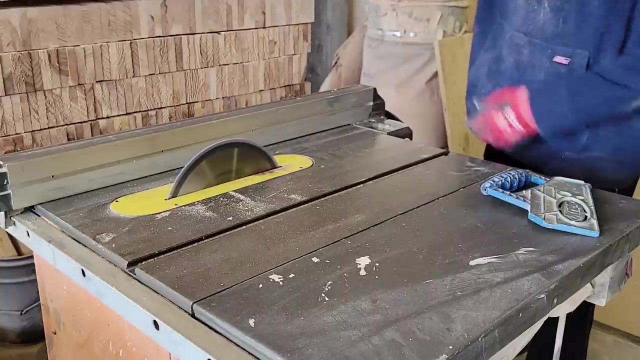 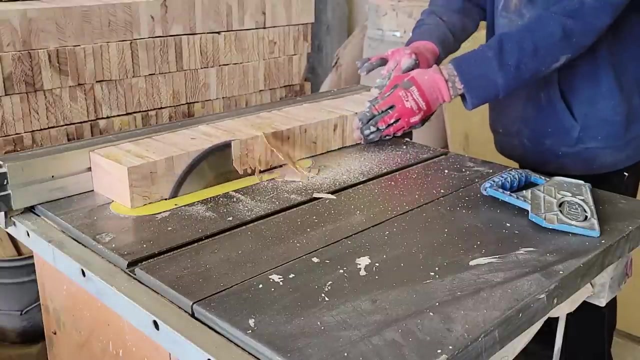 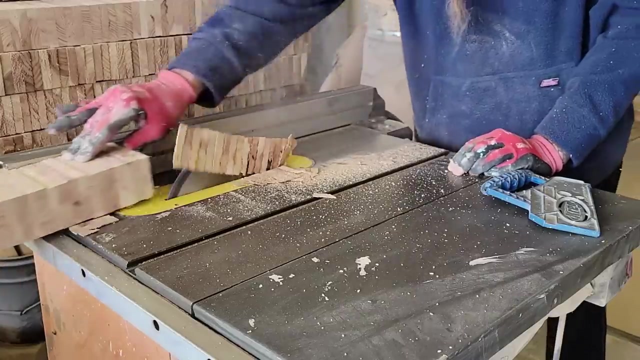 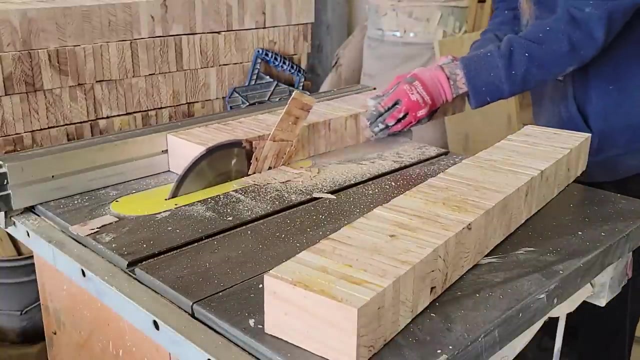 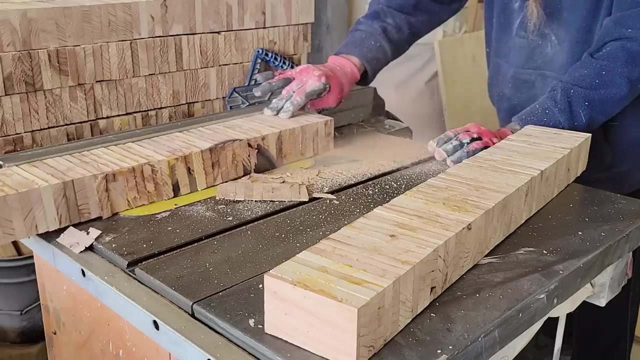 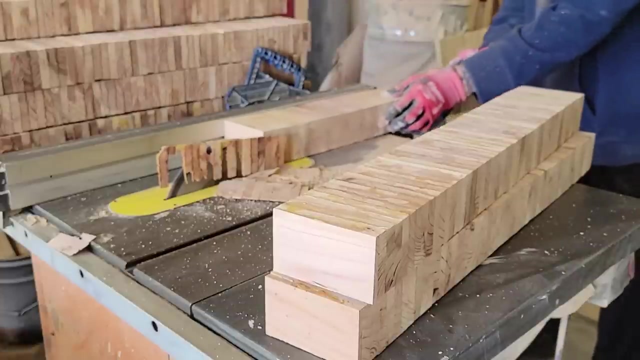 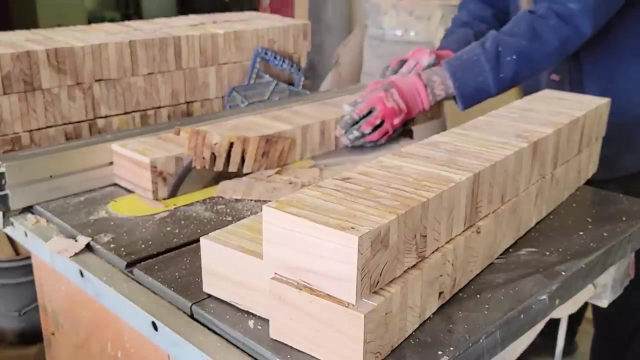 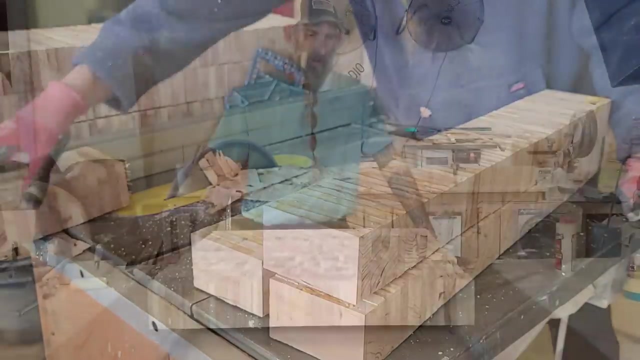 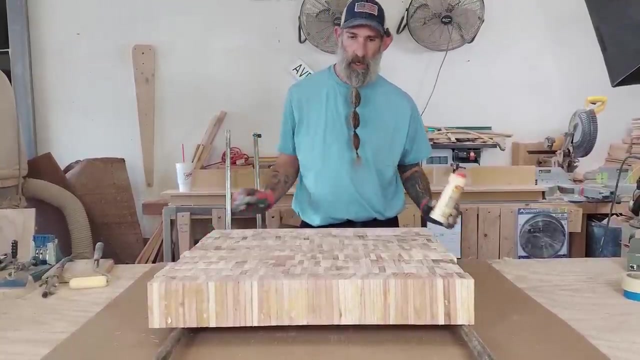 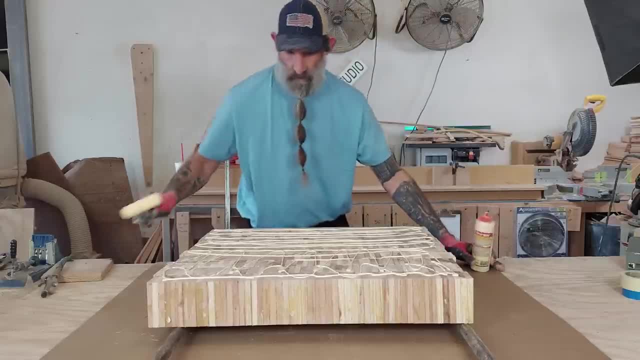 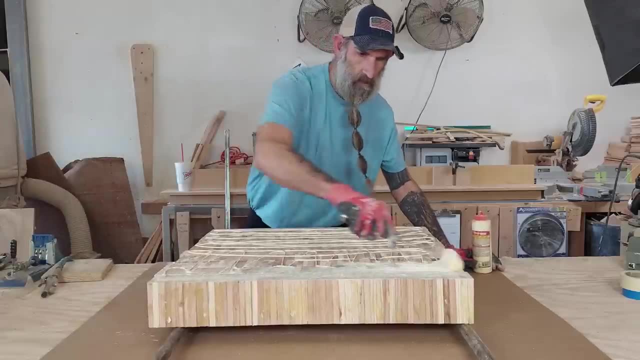 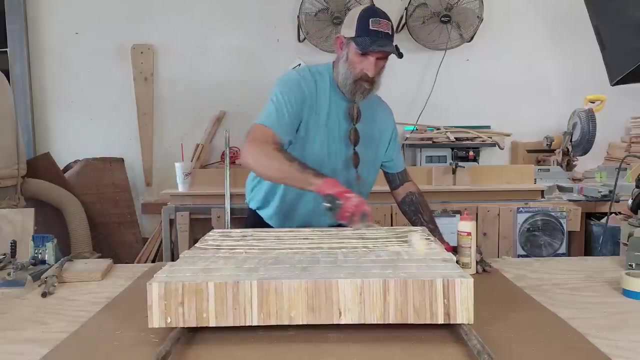 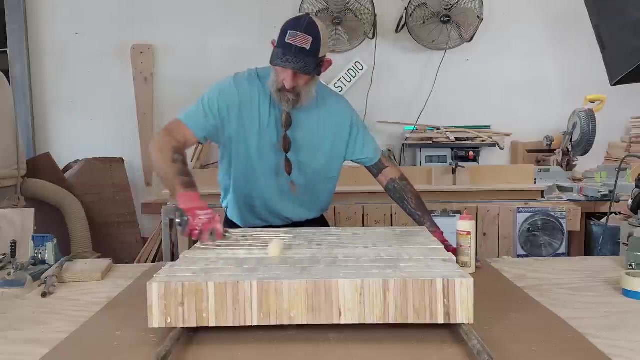 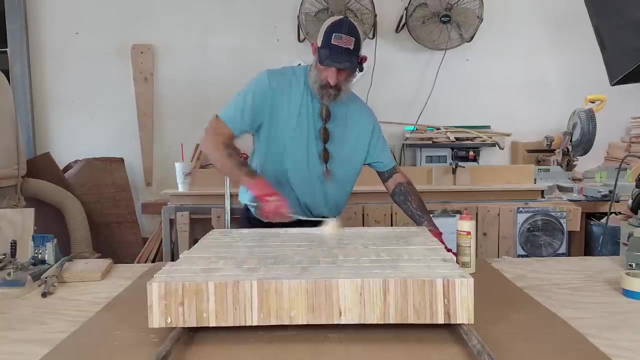 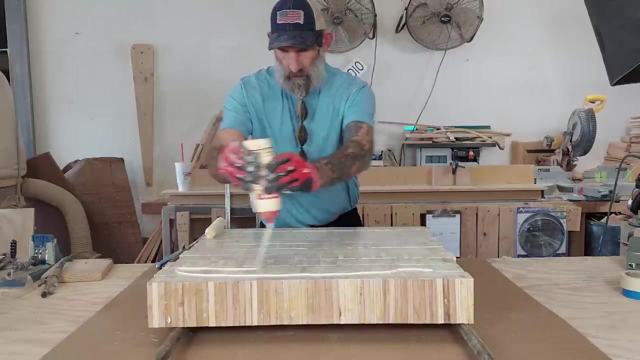 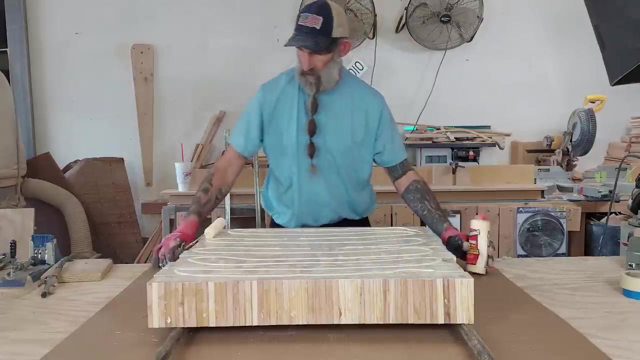 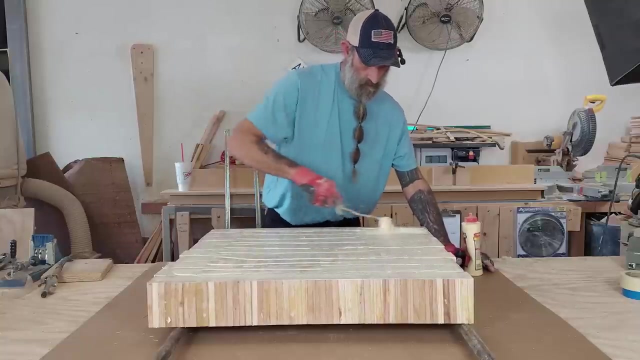 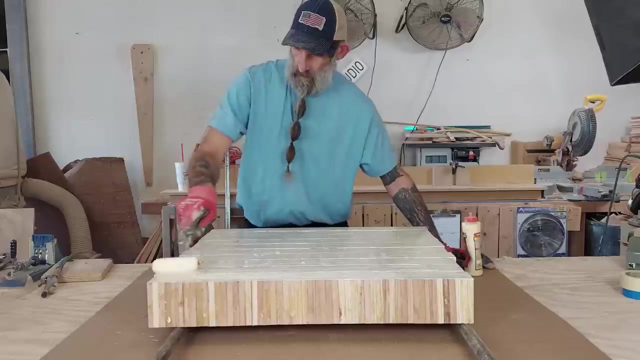 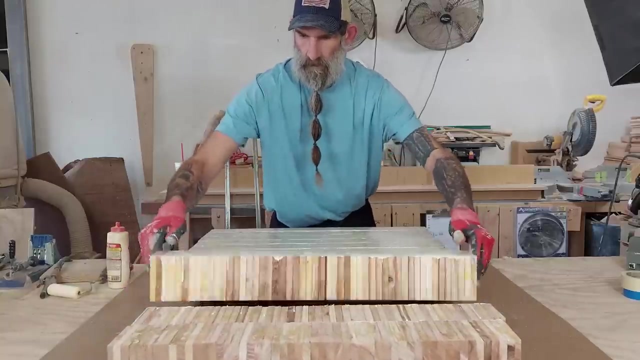 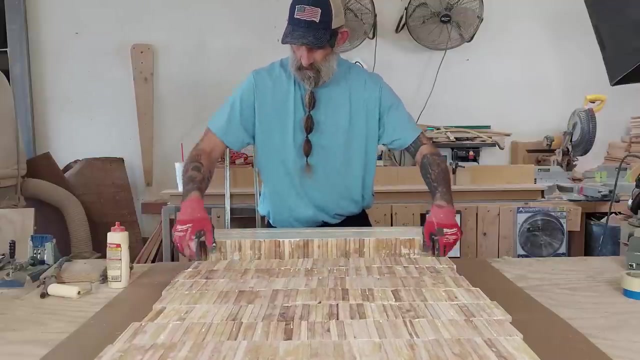 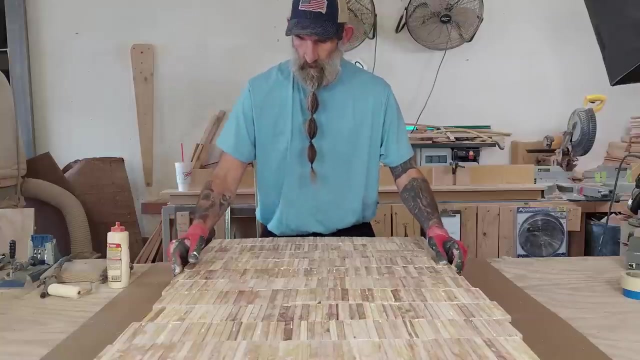 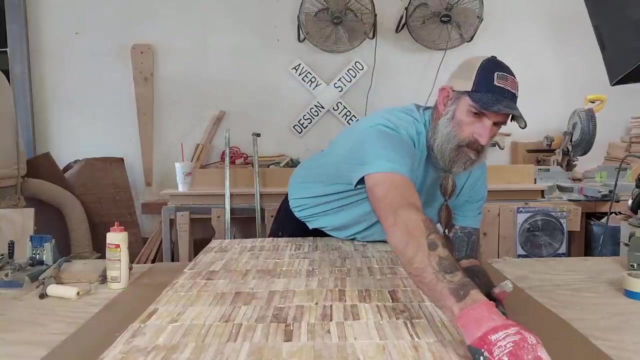 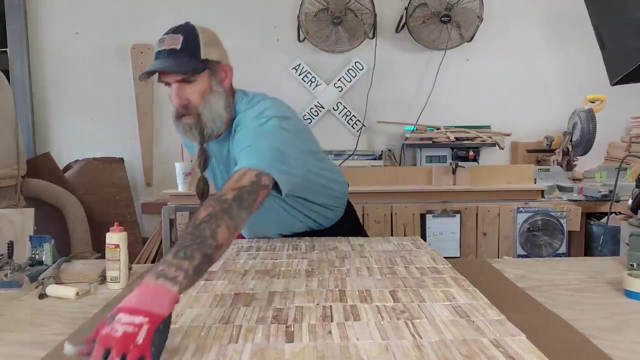 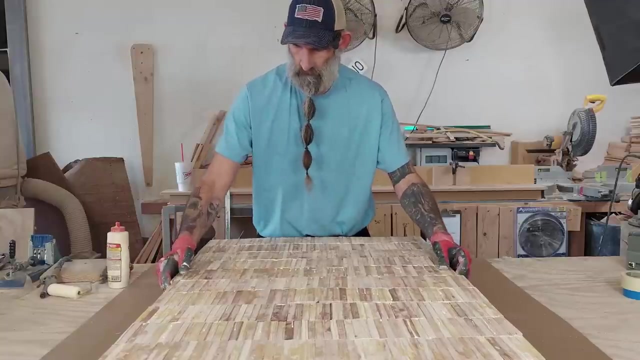 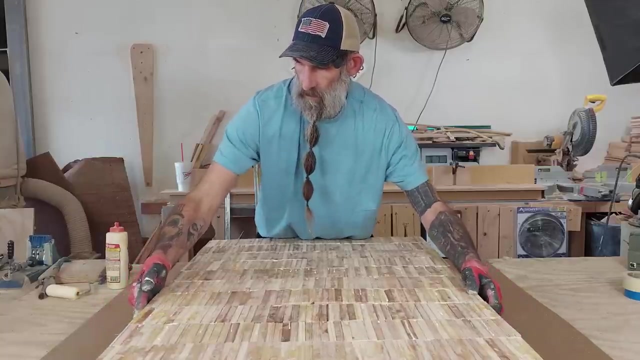 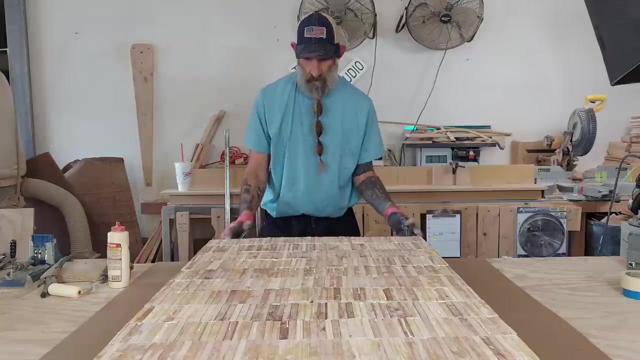 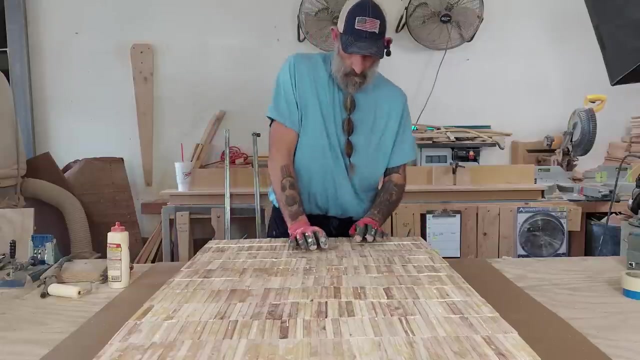 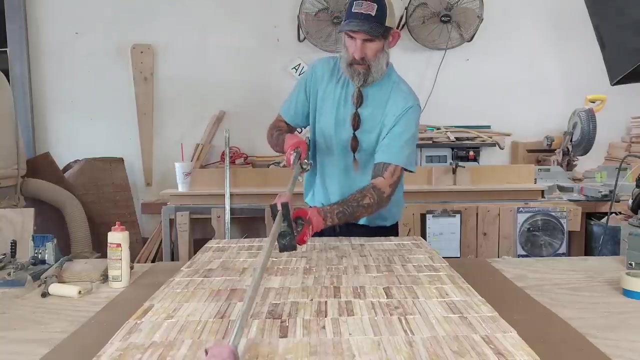 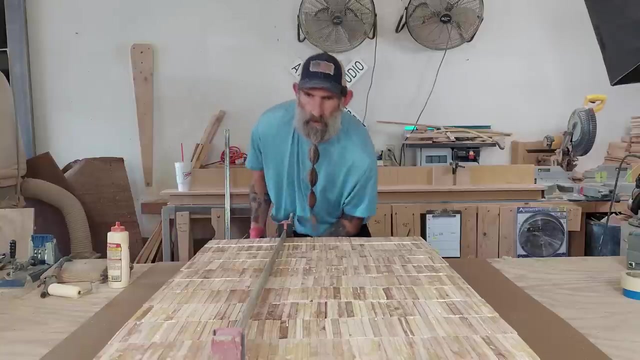 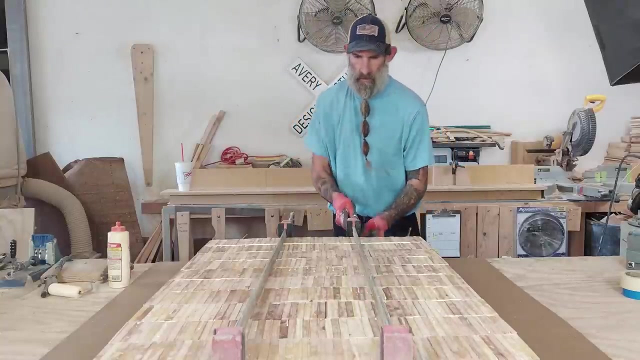 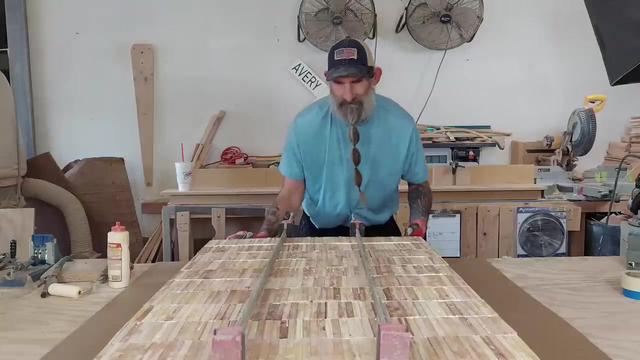 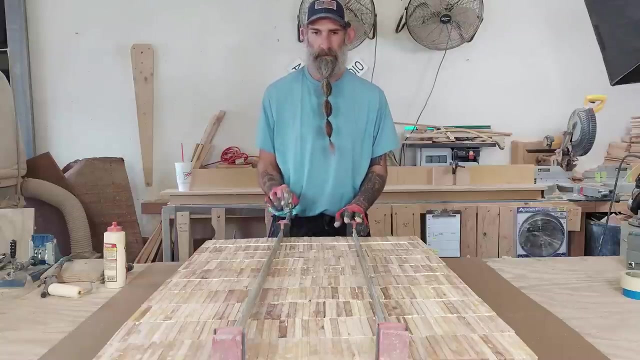 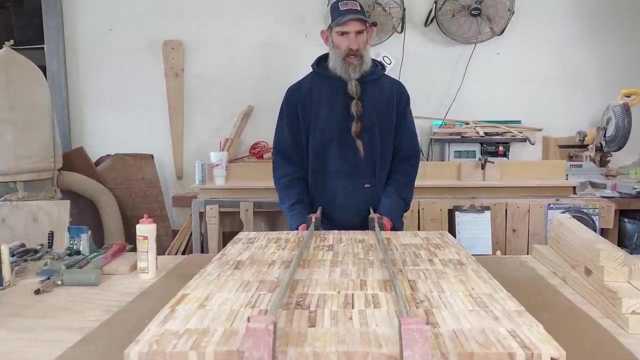 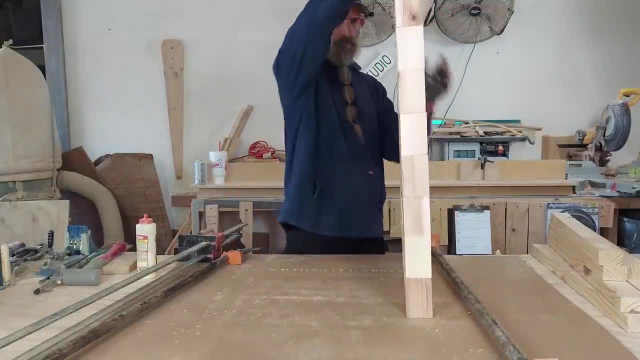 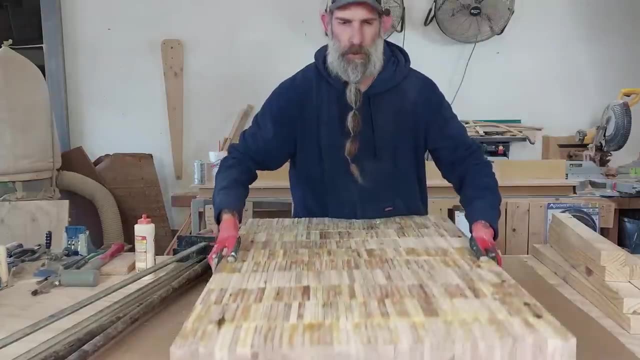 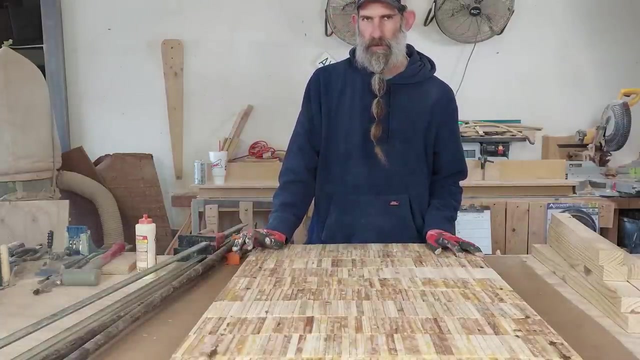 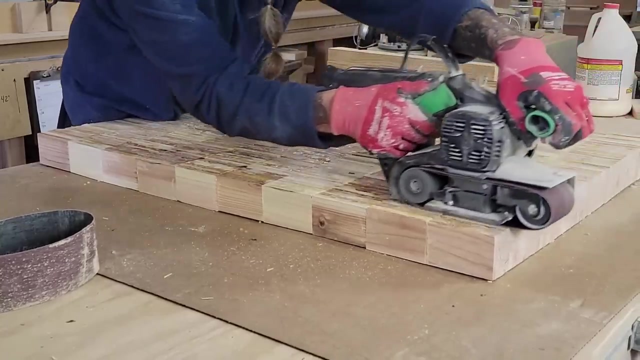 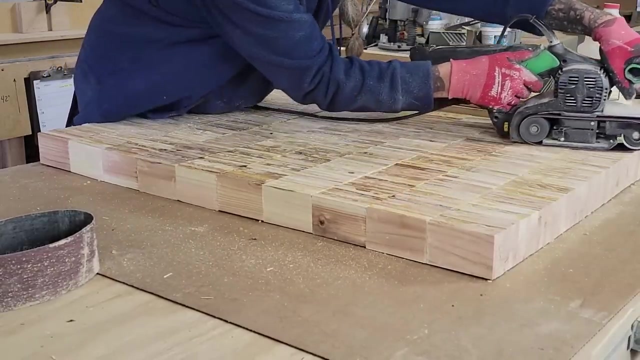 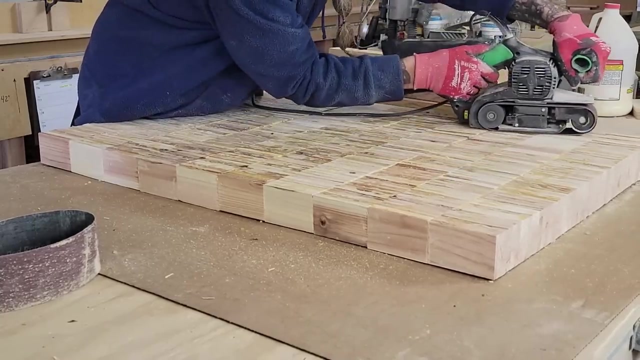 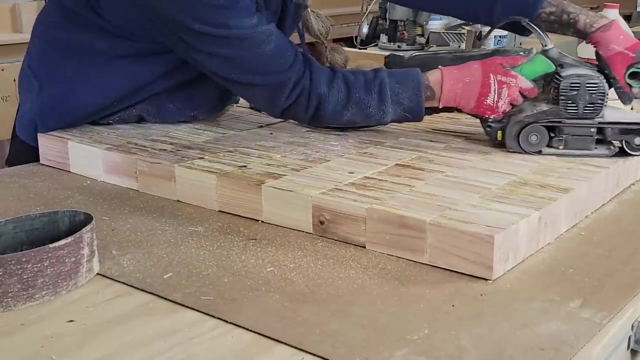 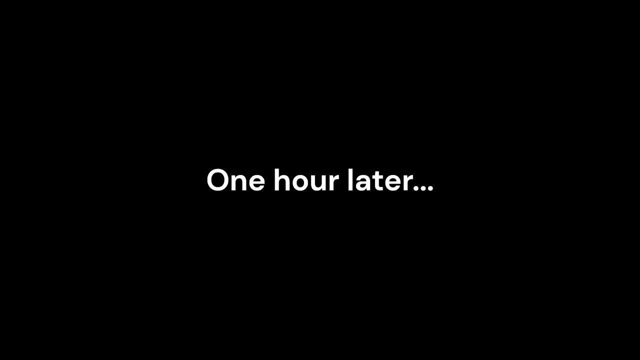 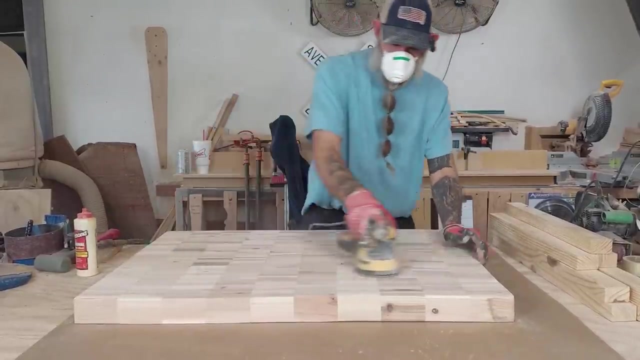 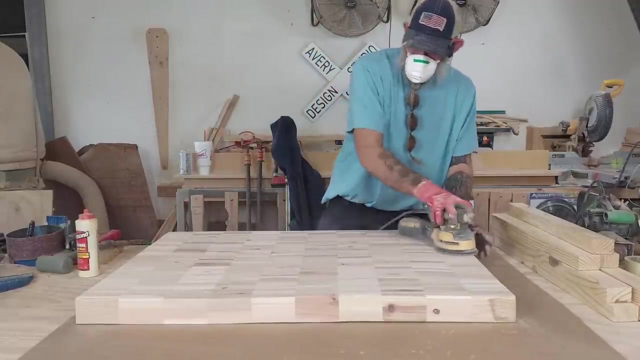 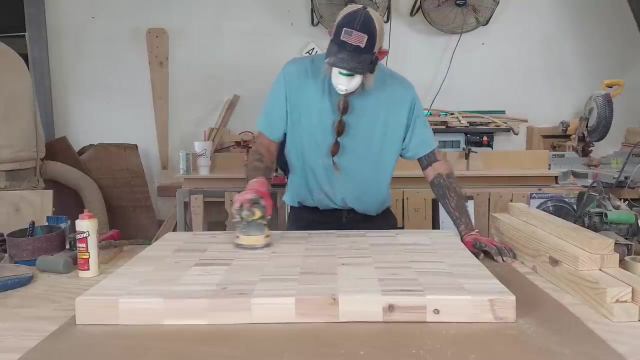 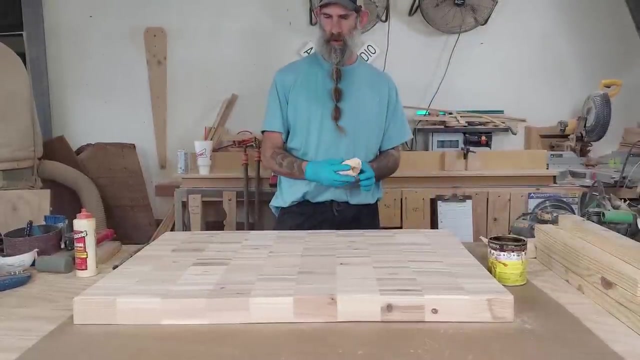 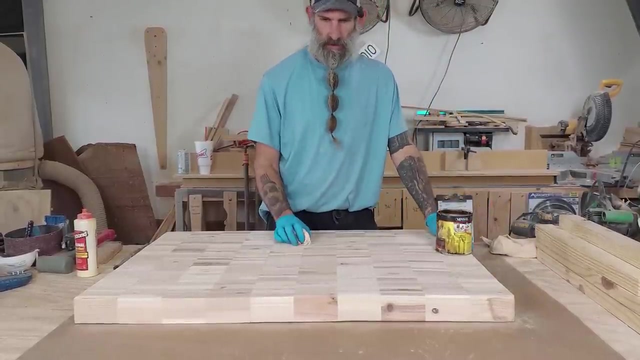 pretty good. uh, now we got a lot of sanding to do, so that's what we're going to do next. so We're going to use this Minwax Early American color on it so it doesn't turn out too dark. So we're going to go ahead and stain it and let it dry, and then we'll do the legs after that. 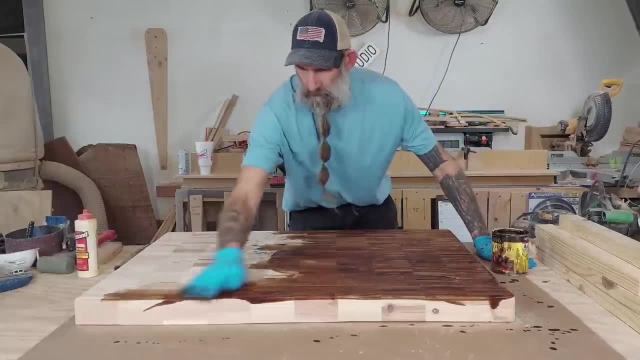 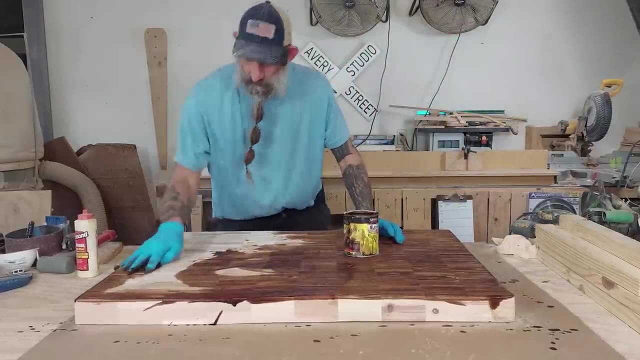 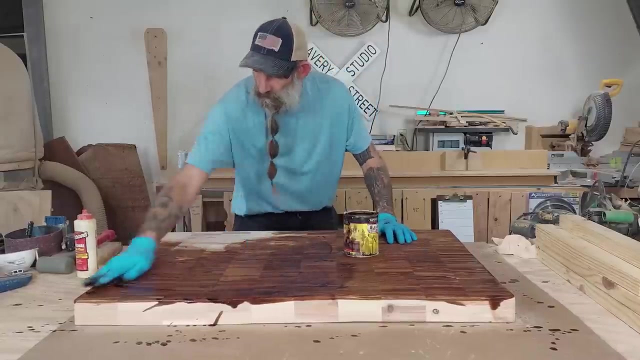 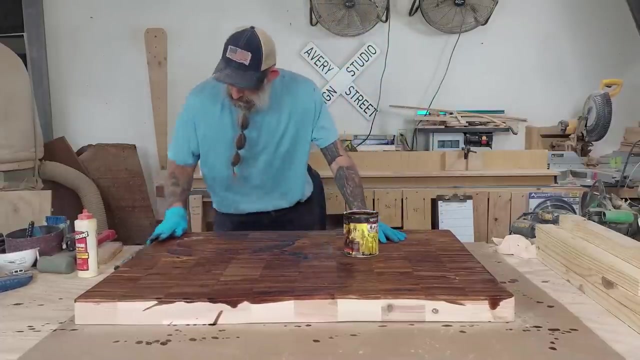 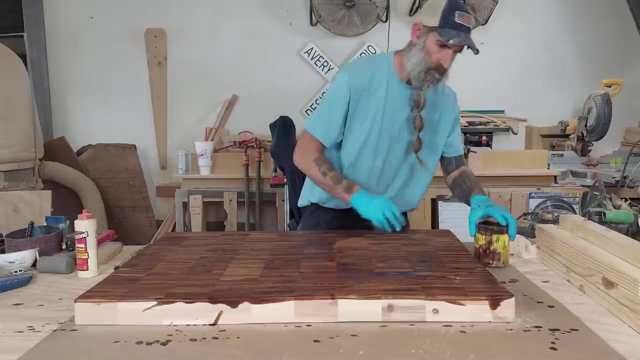 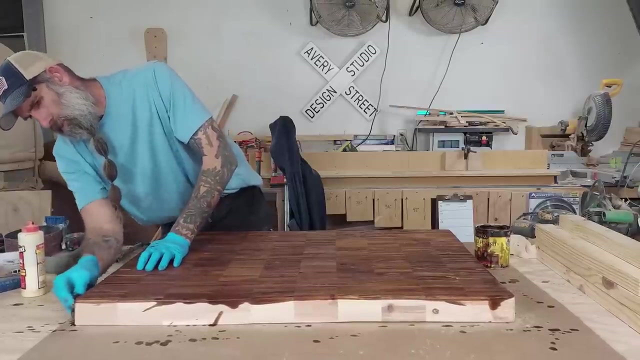 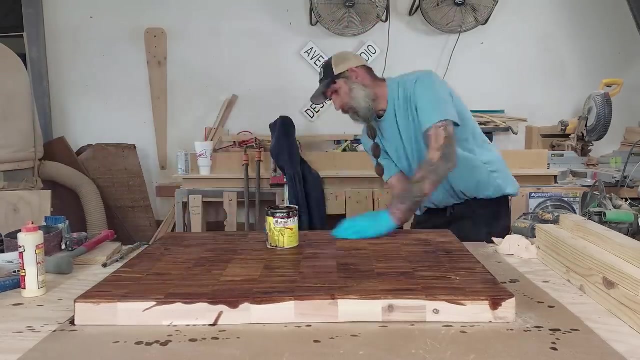 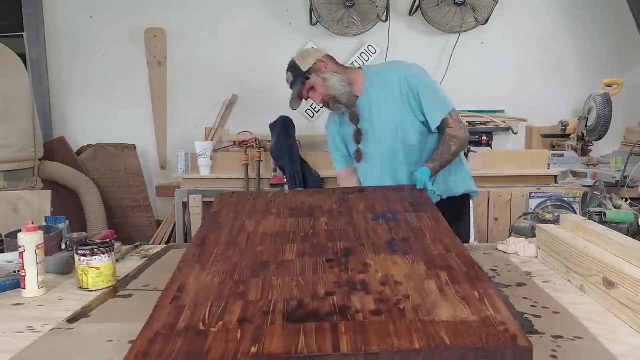 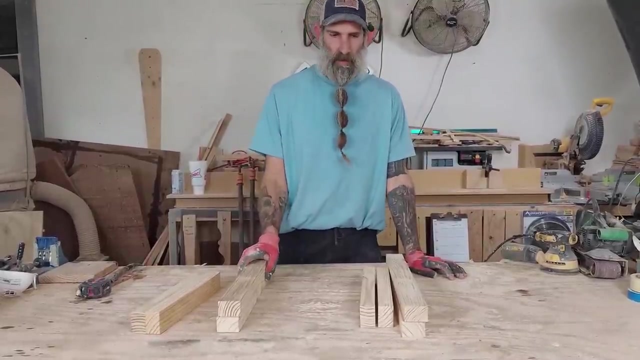 So we're going to go ahead and stain it and let it dry. So we're going to go ahead and stain it and let it dry. So now we're going to do the legs. These are cut-offs from our shelves that we make. 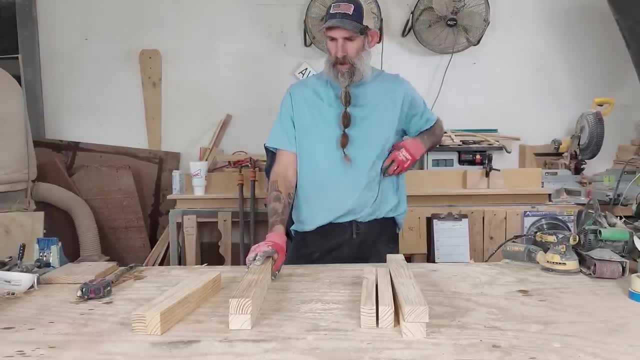 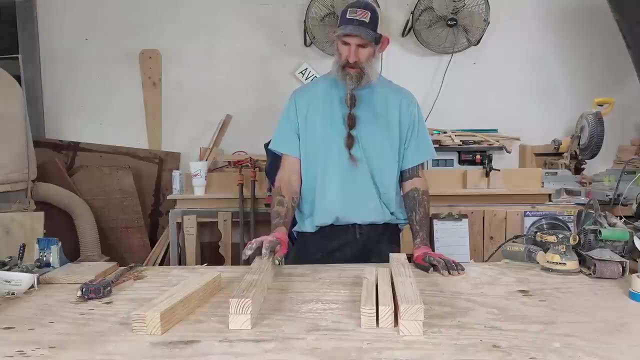 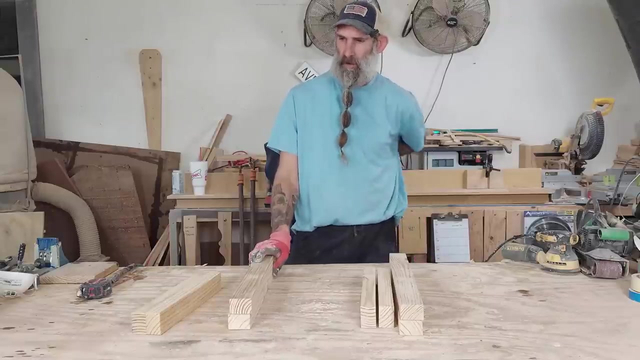 So this entire table is completely free. We put zero money into it And we're going to make faux metal tubing square legs out of these cut-off pieces of 2x10.. So I'm going to drill some pocket holes and we'll screw it all together and get them painted. 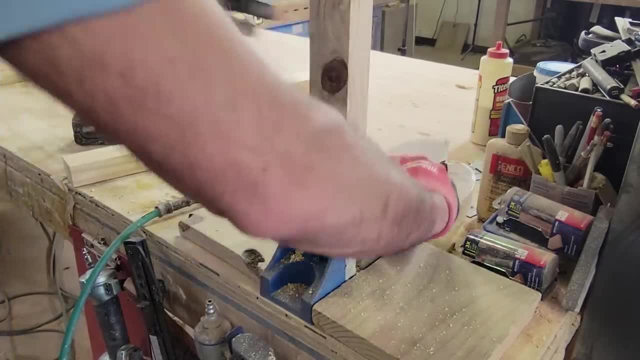 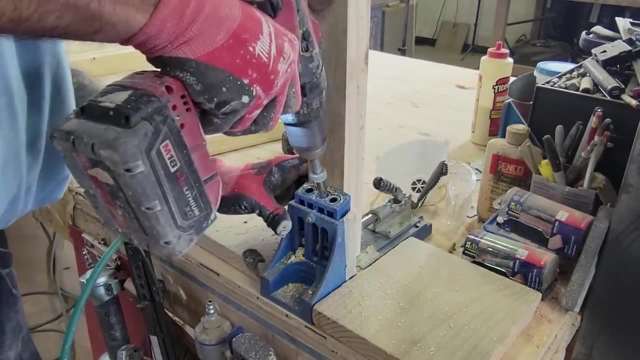 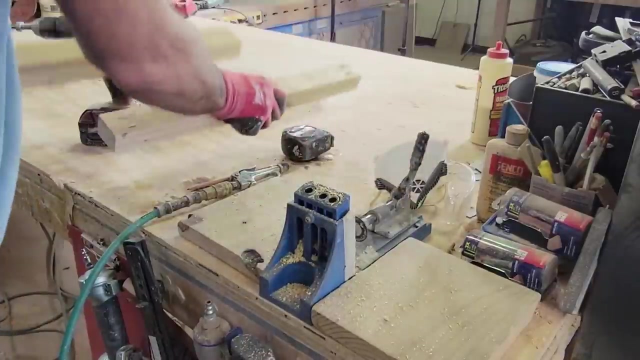 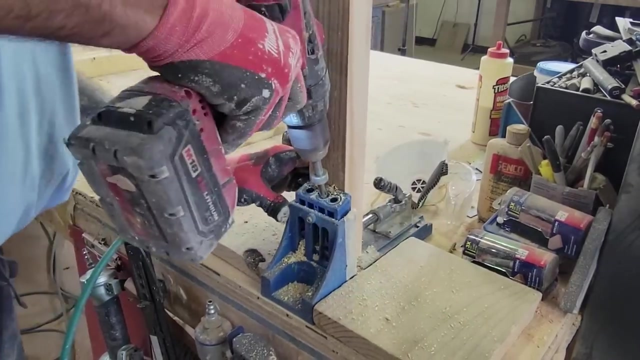 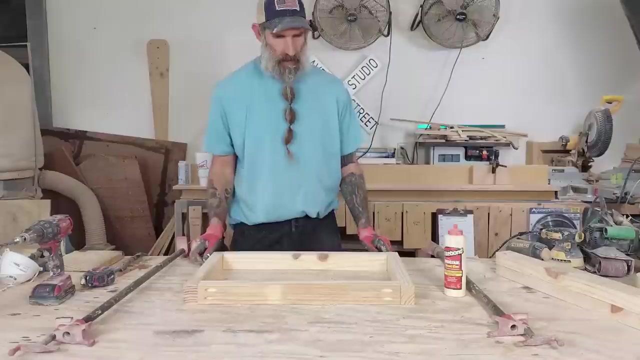 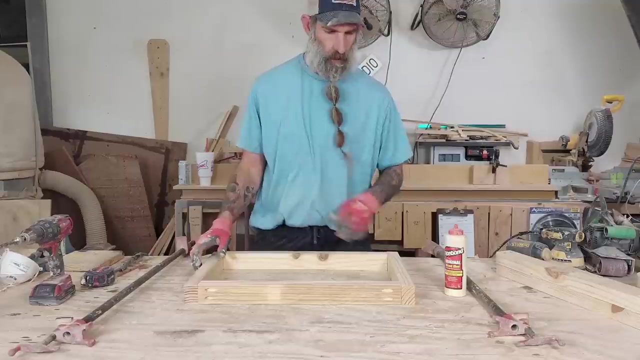 So I'm going to drill some pocket holes and we'll screw it all together and get them painted. So now we've got all the pocket holes drilled and we're going to assemble the legs. I'm just going to glue and clamp and screw them together. 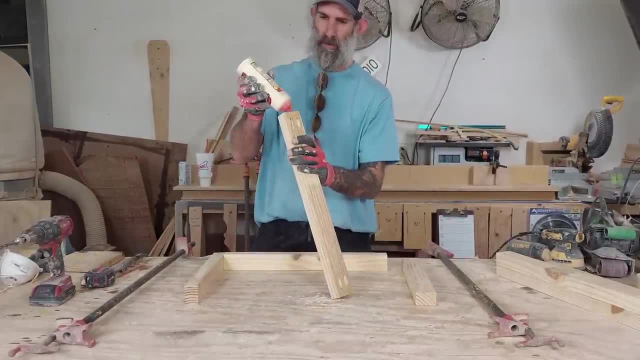 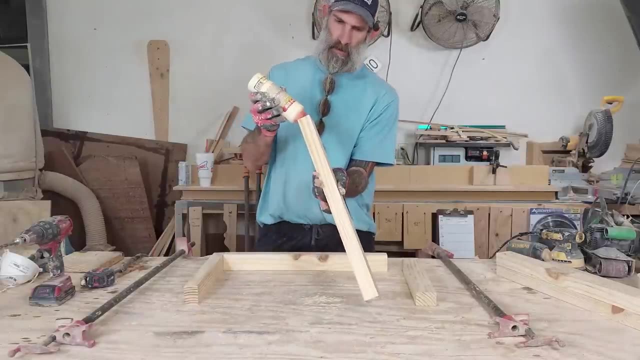 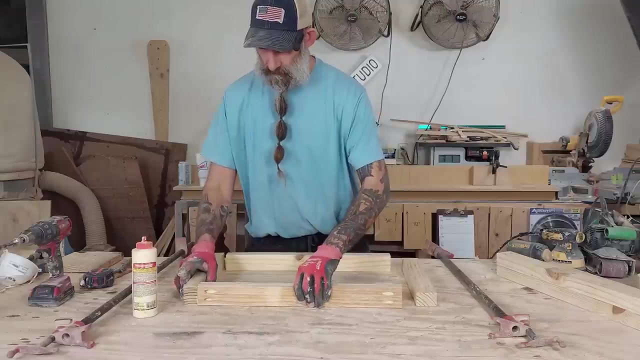 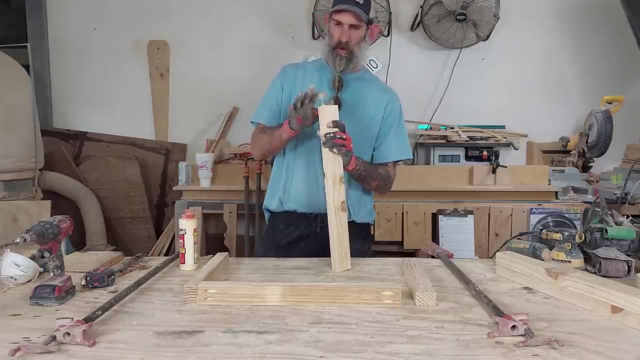 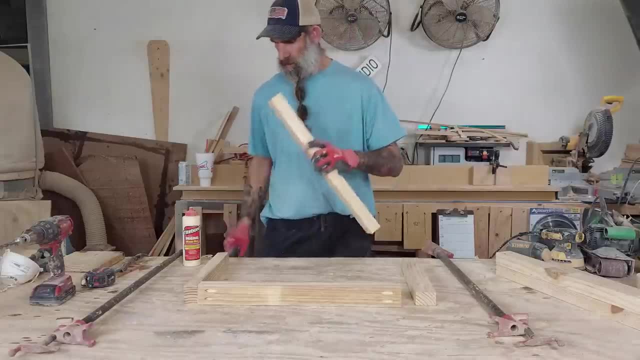 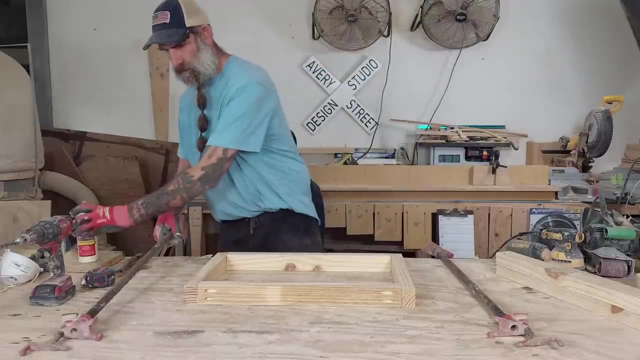 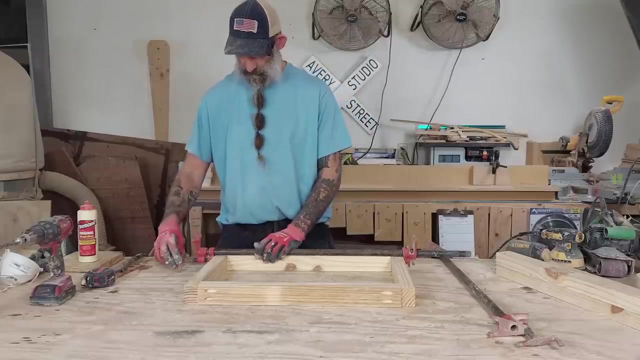 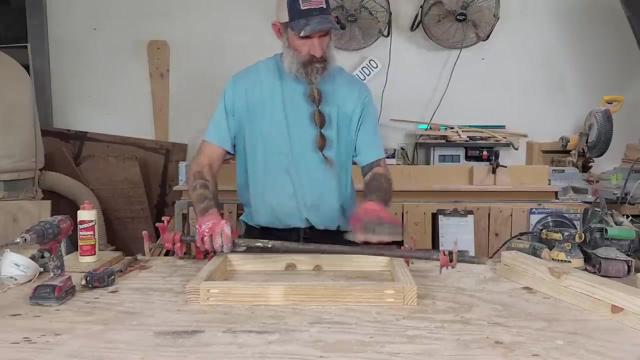 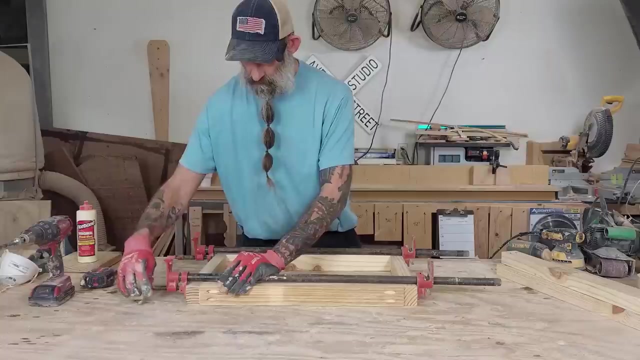 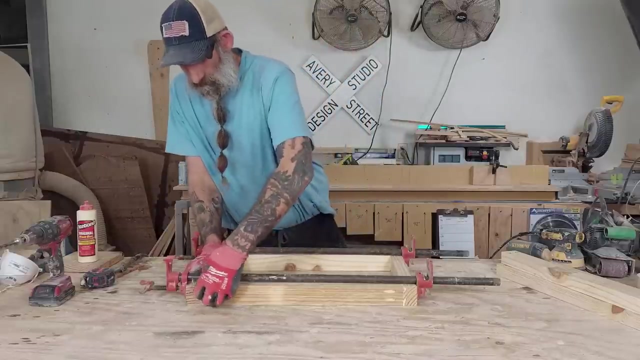 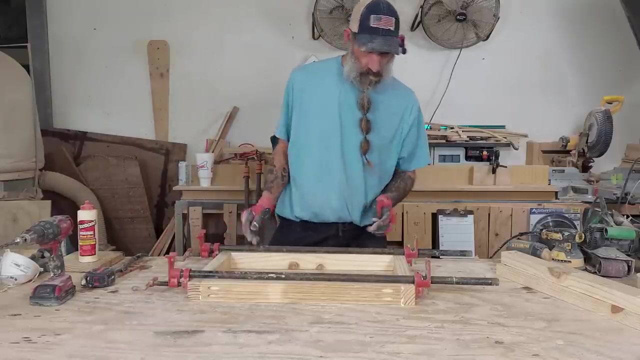 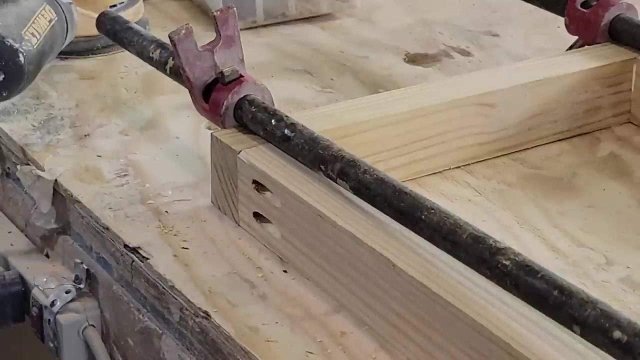 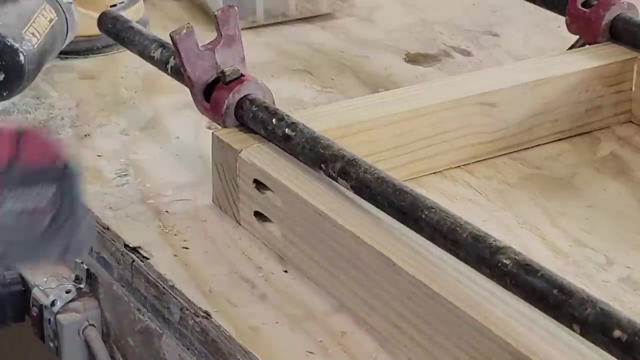 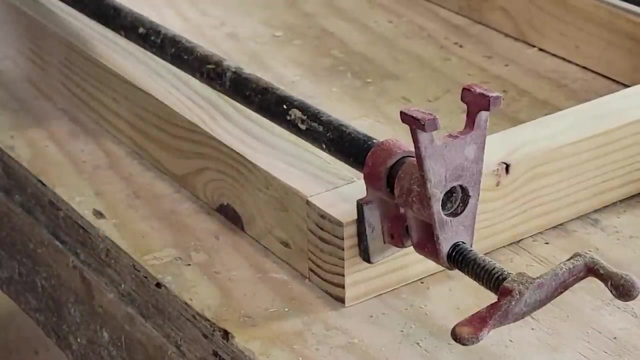 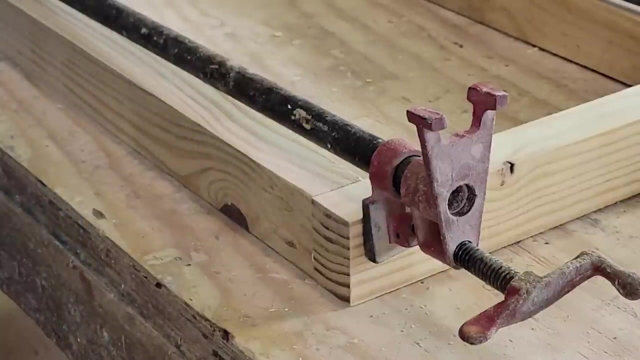 I'm going to put the pocket holes on the top and bottom so they're not visible. I'm going to put the pocket holes on the top and bottom so they're not visible. Let's go, Let's go, Let's go. So now I got both the legs sanded, ready for paint. 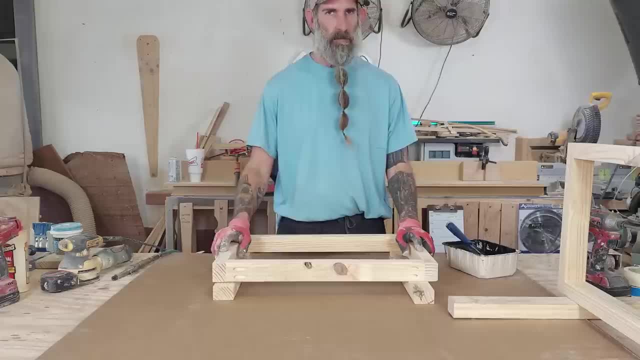 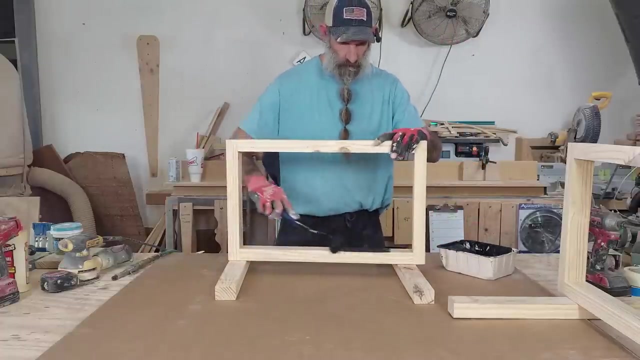 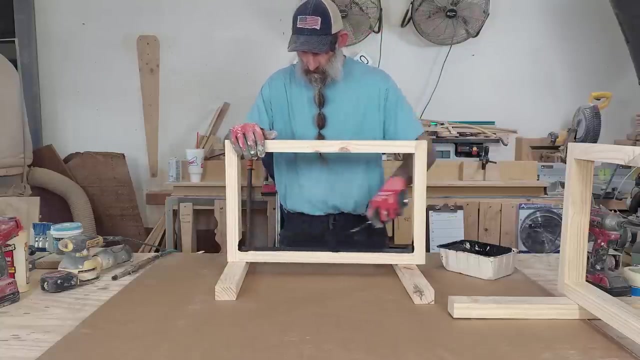 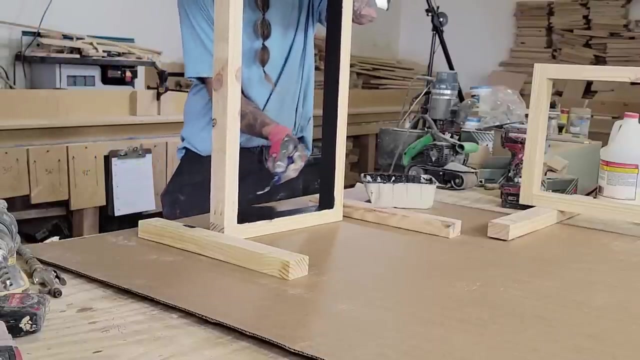 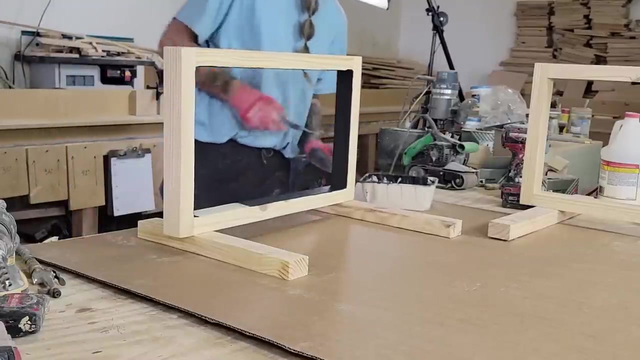 I'm going to go ahead and put two coats of black paint on each of the legs and then they'll get sprayed with the sealer. At the same time I'm spraying the table. I'm going to go ahead and spray the table. 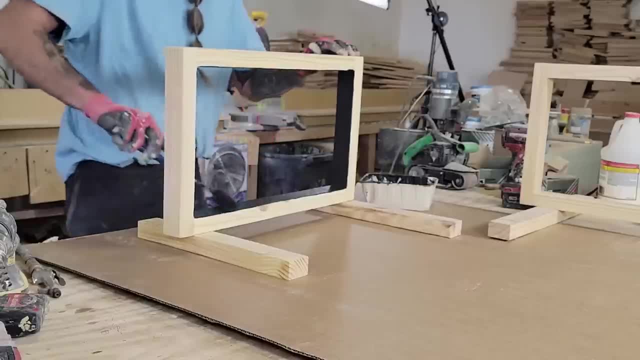 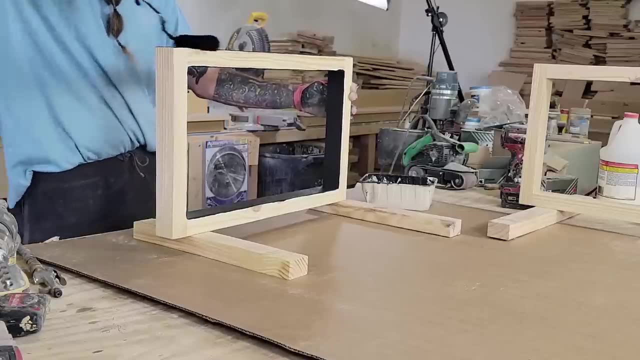 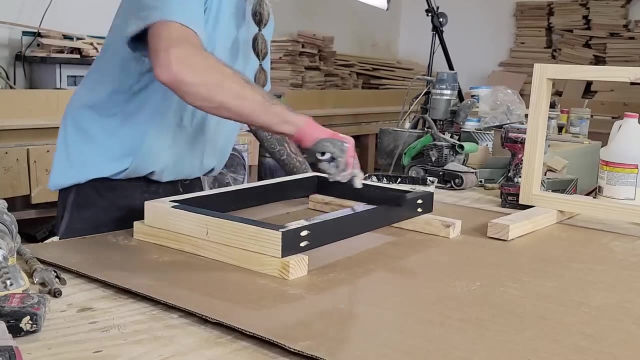 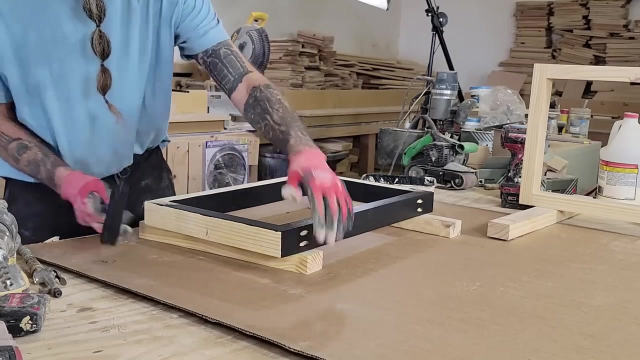 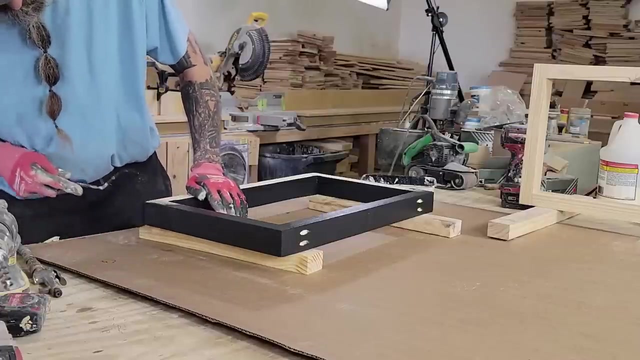 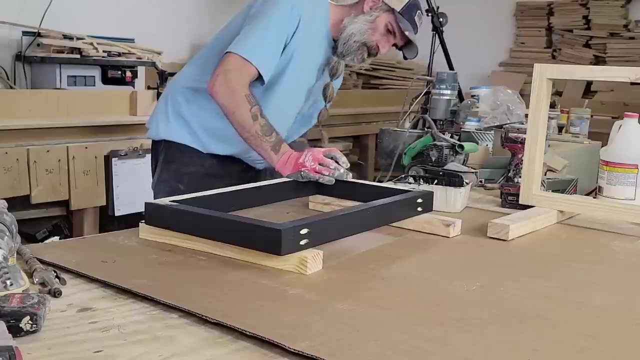 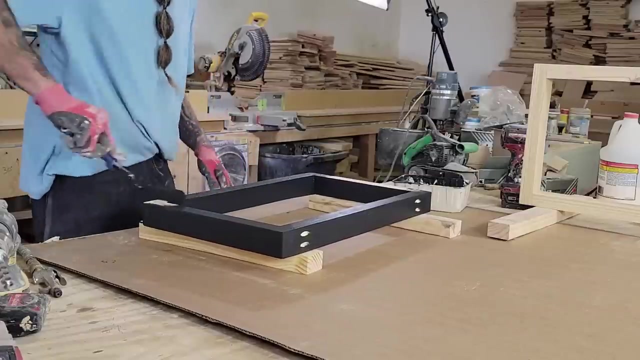 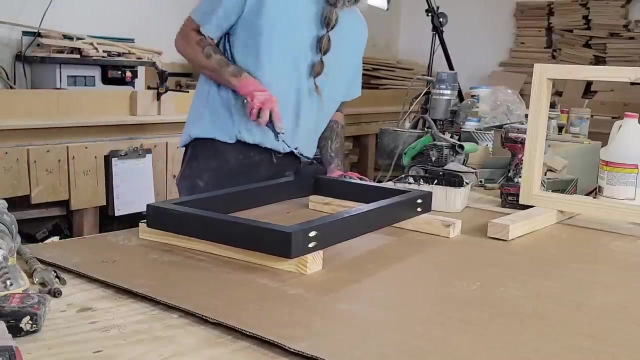 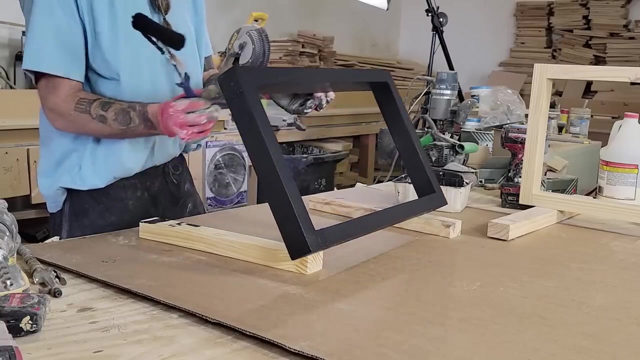 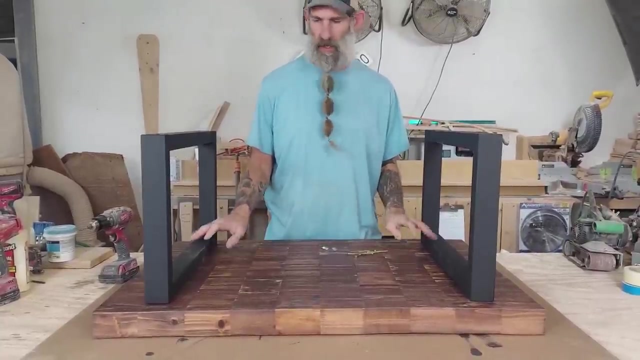 I'm going to go ahead and spray the table. I'm going to go ahead and spray the table. So now I've got the table stained and sealed. I've got the legs built and painted. I'm going to attach the legs to the bottom of the tabletop. 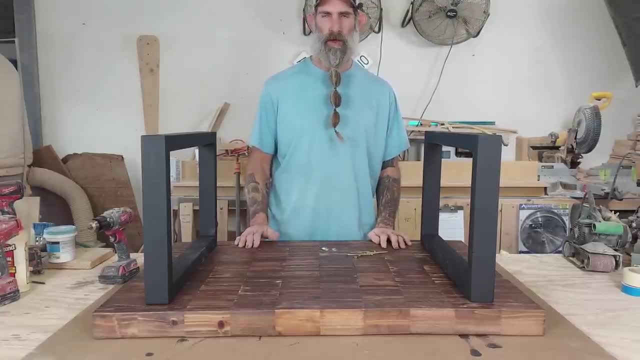 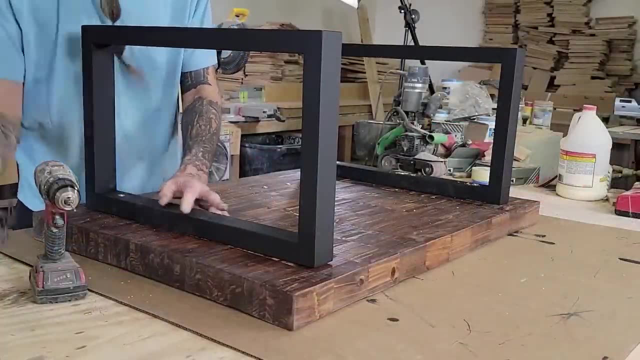 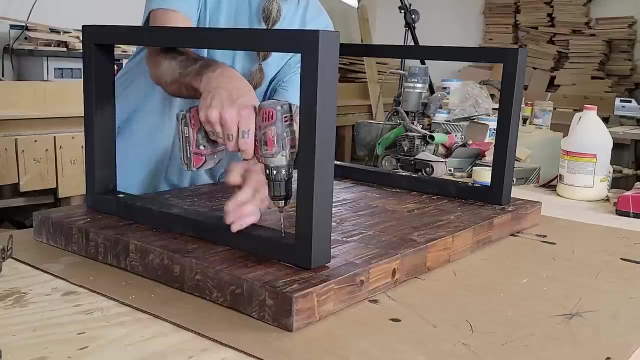 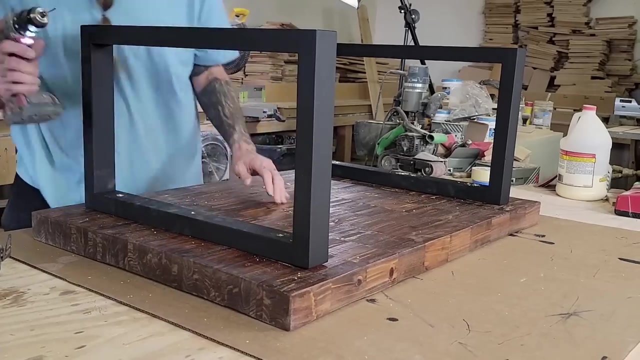 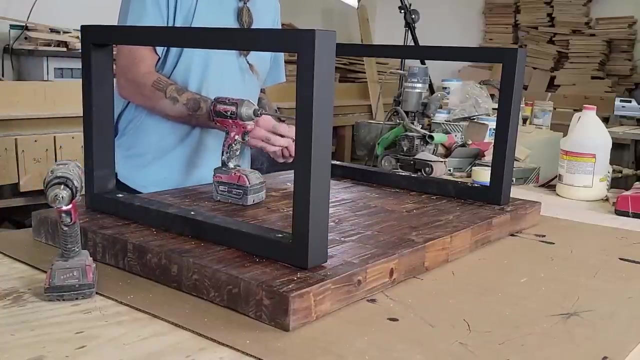 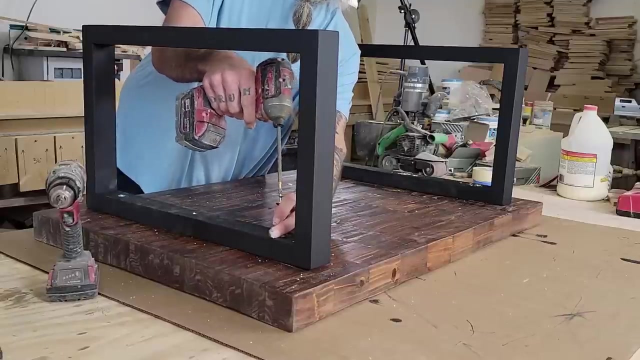 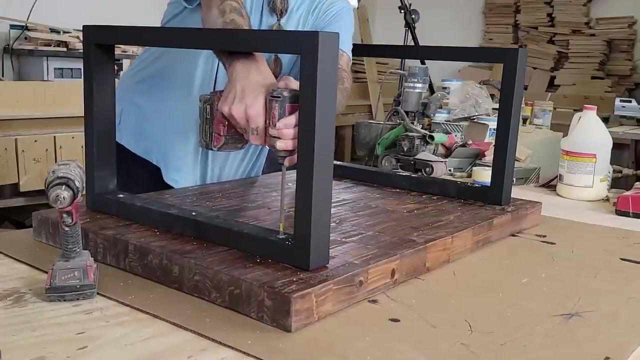 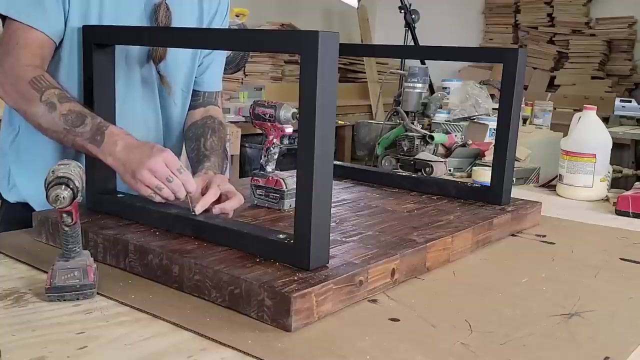 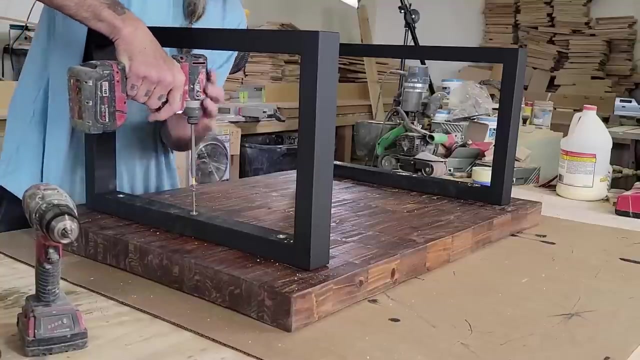 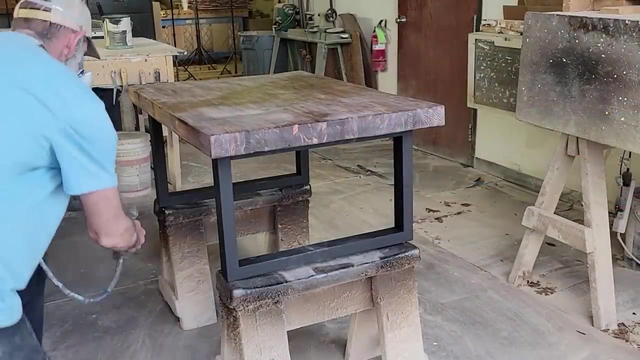 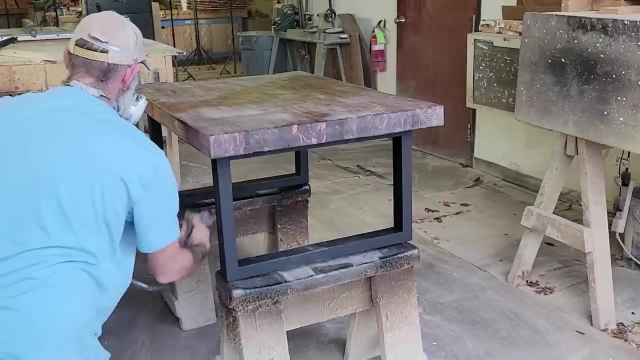 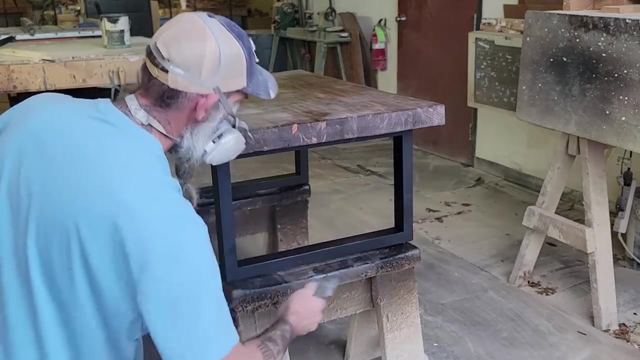 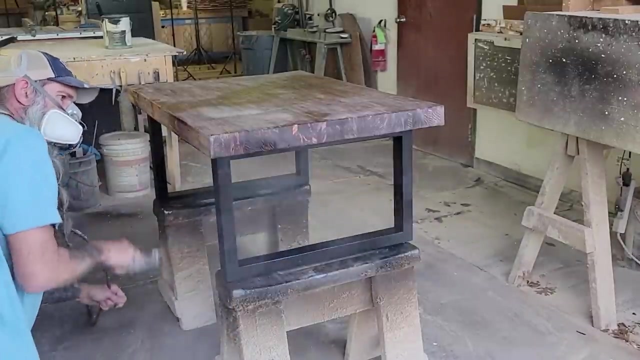 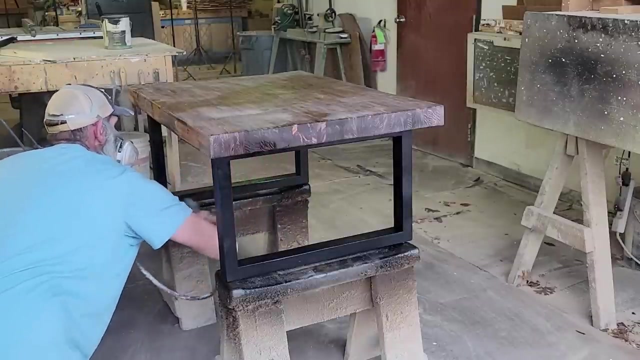 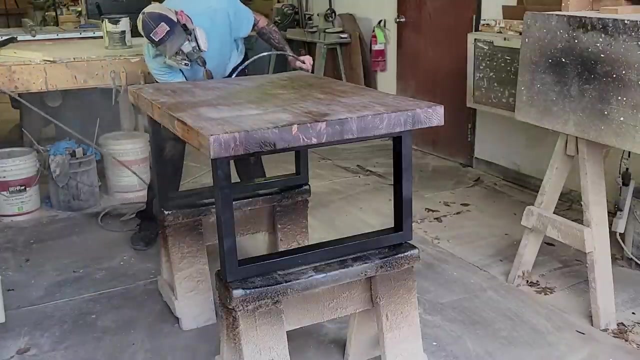 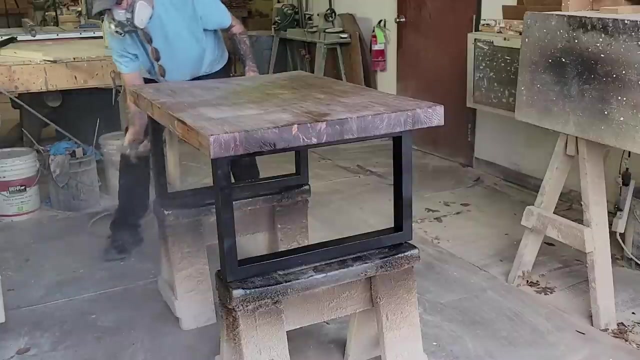 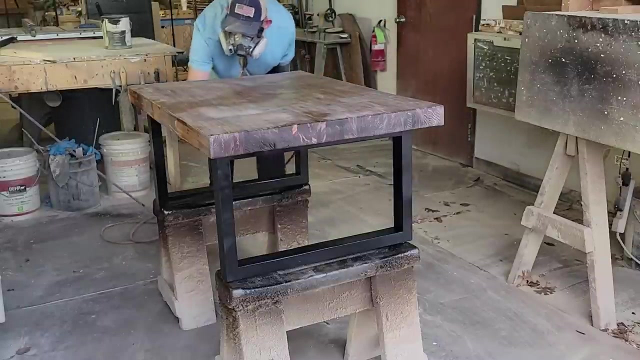 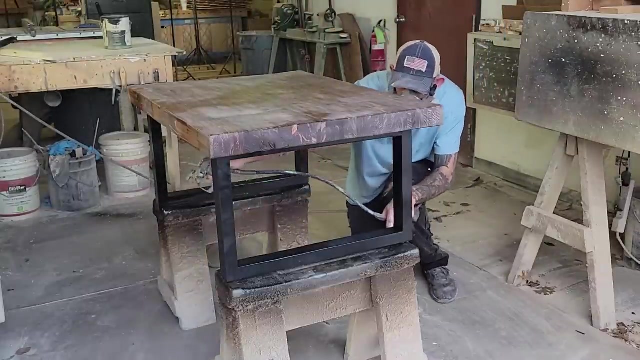 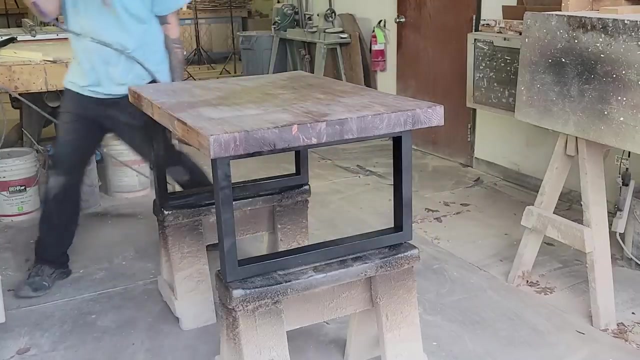 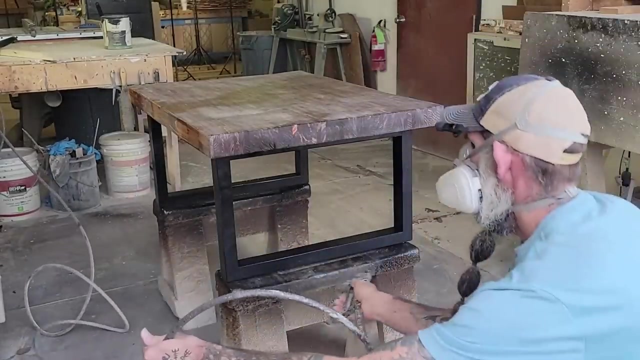 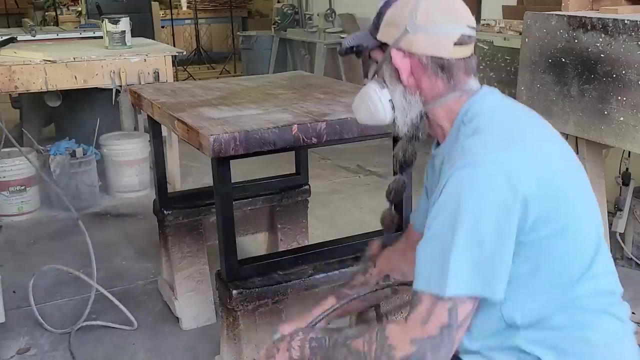 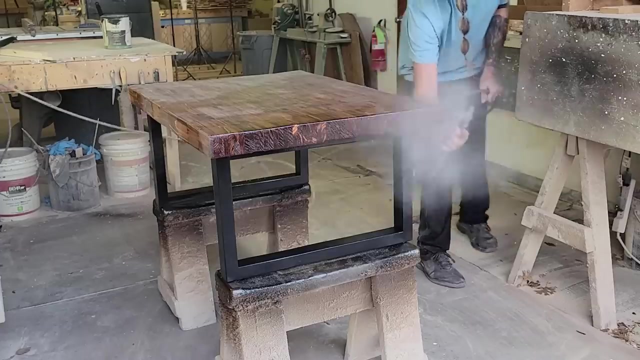 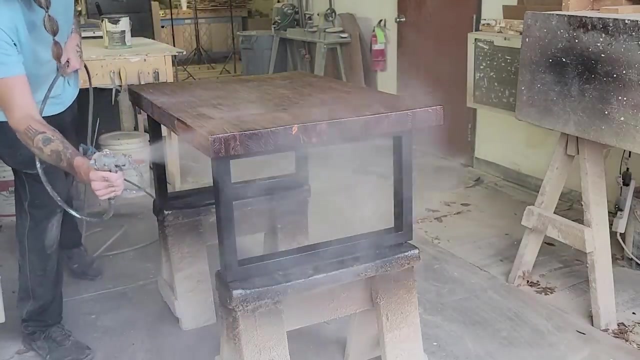 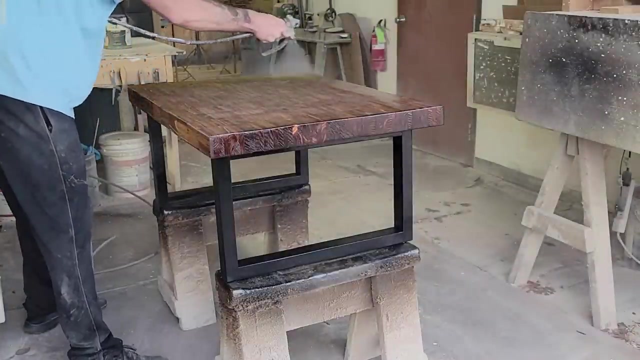 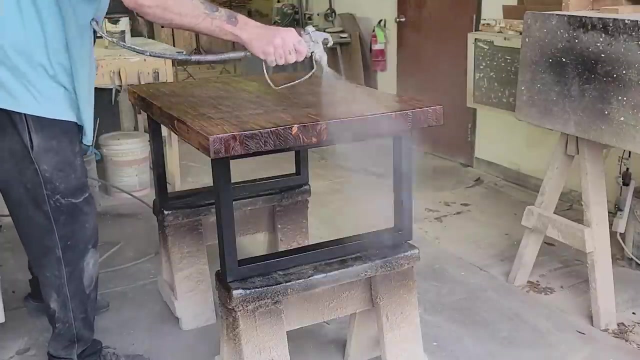 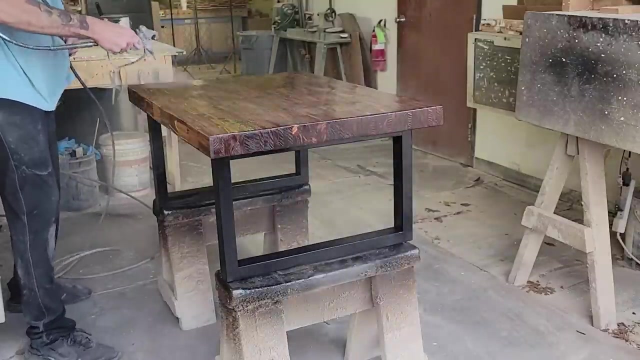 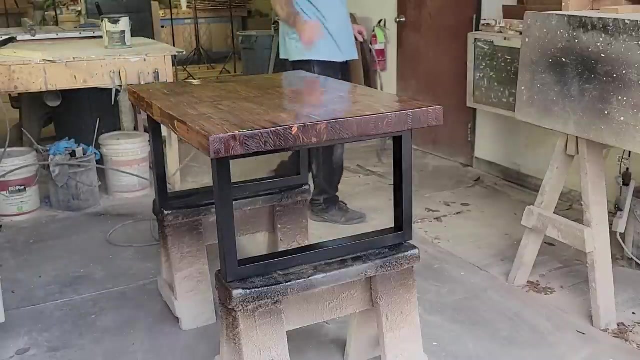 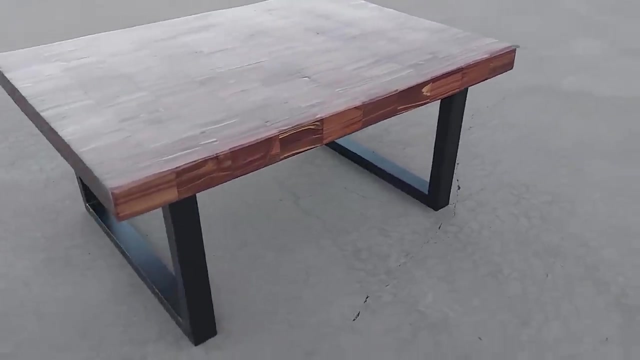 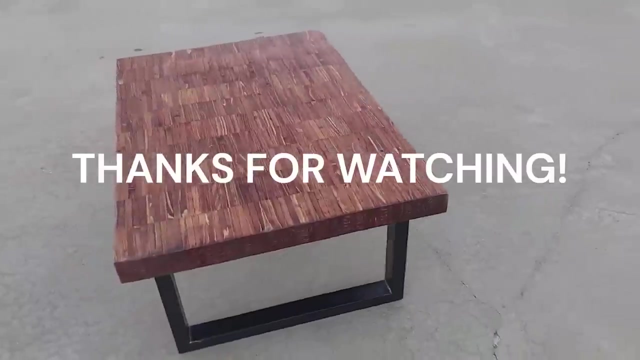 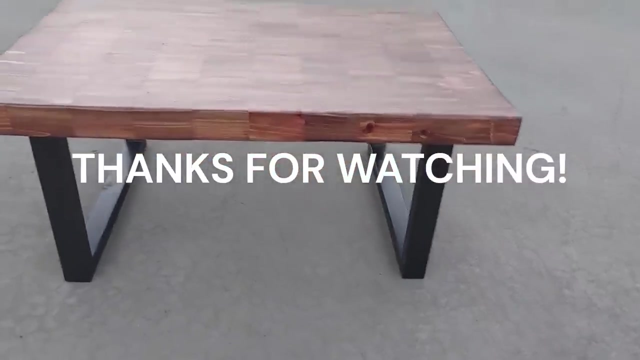 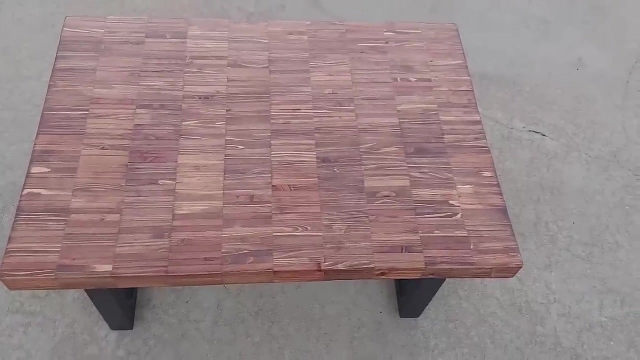